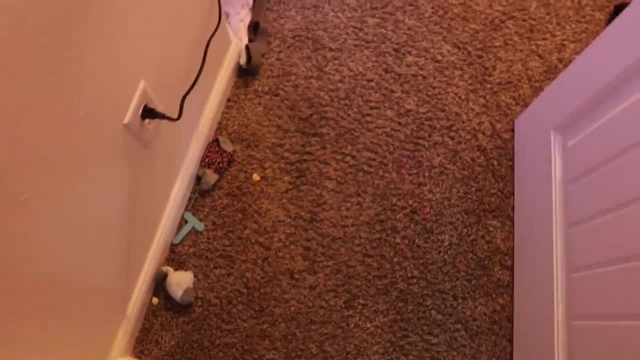 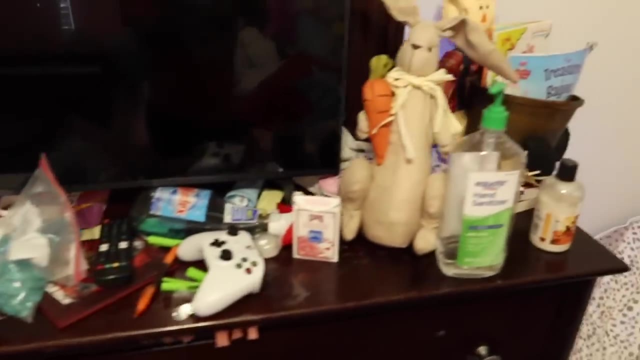 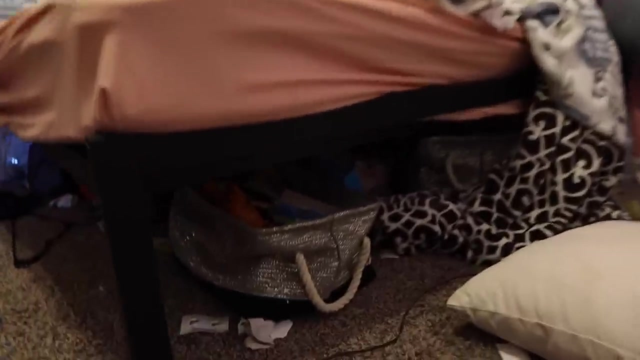 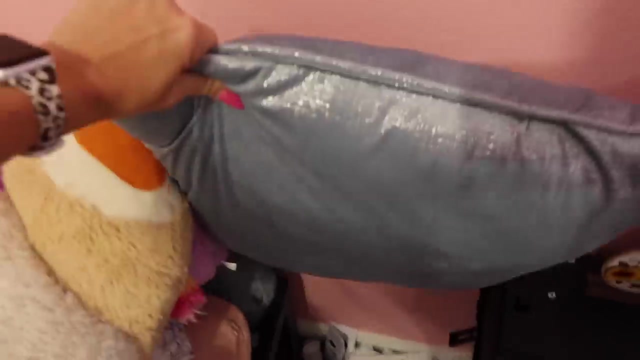 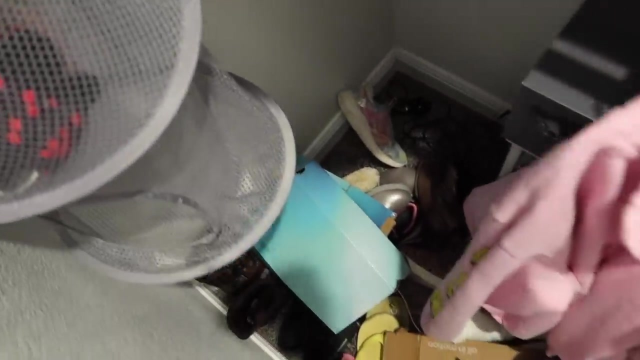 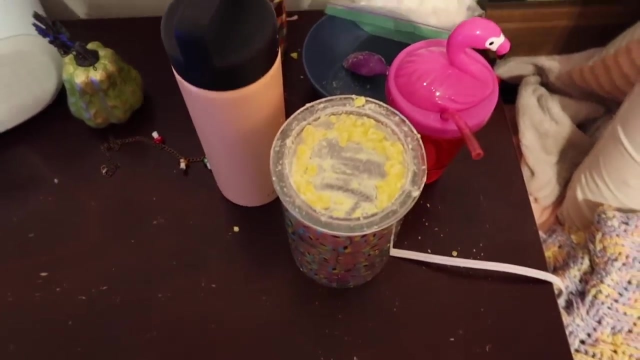 leave that, since she likes it. but you guys, this is what her room is looking like. I've been looking for my pillow. she had it. I'm thinking about the days we used to shine when we were young. I told you that. what in the actual world? 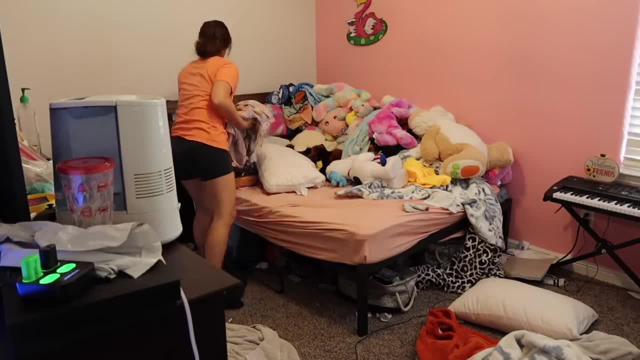 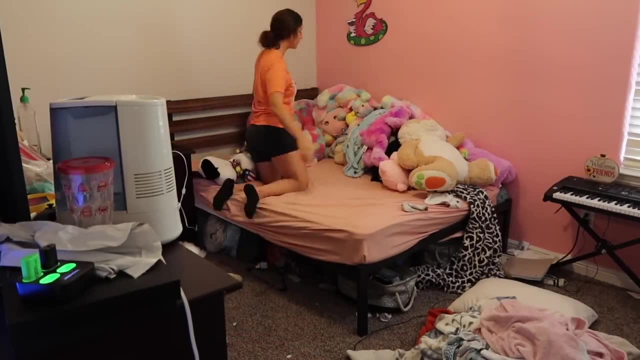 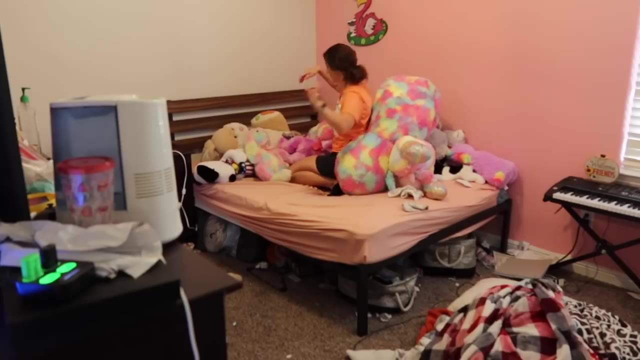 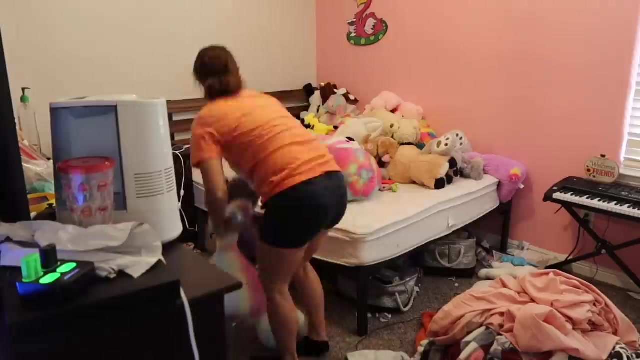 it's 2 am and I can't fall asleep. I'm just not tired. I can hear the raindrops falling, it's cold outside and I kind of feel like calling, but it's too late now. I just miss you. so y'all. my child has a serious blanket hoarding problem. 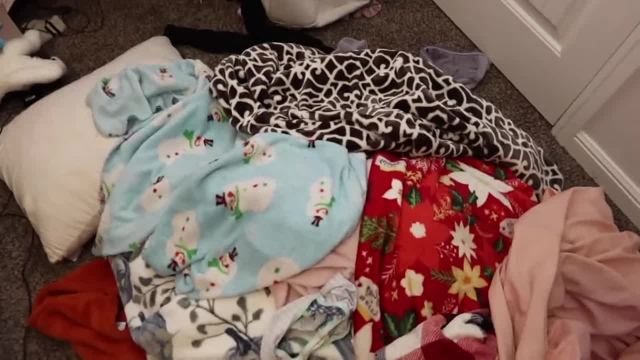 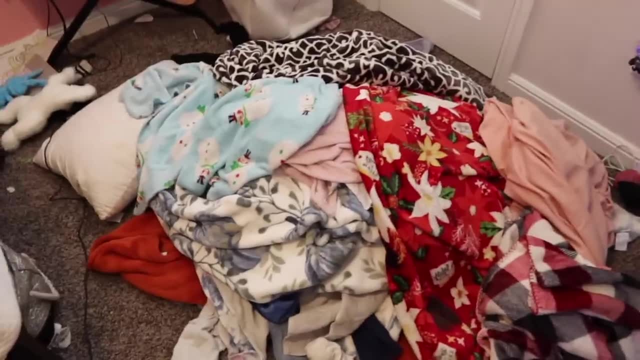 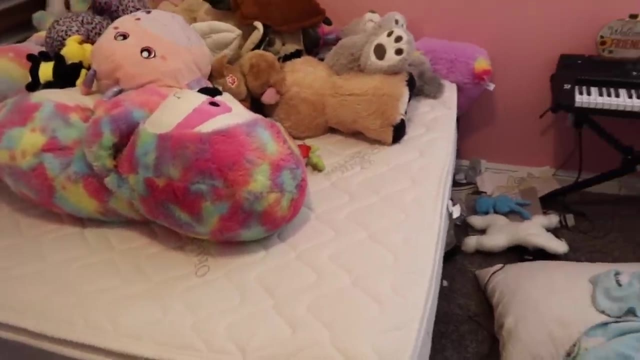 this is like probably 75% of all the blankets we own. it was all in her bed, so we're gonna go ahead, wash these. I'm gonna spray all the stuffed animals down and her mattress with the Odo band just to help disinfect, and all of that as you. 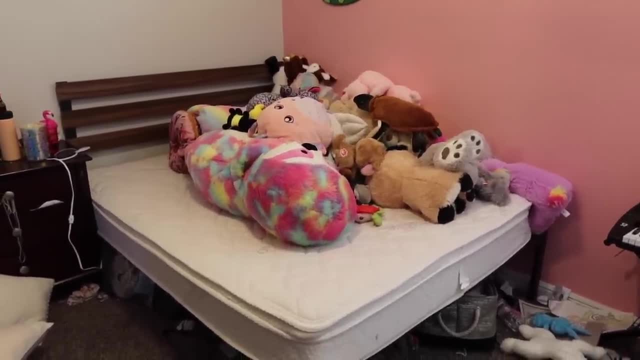 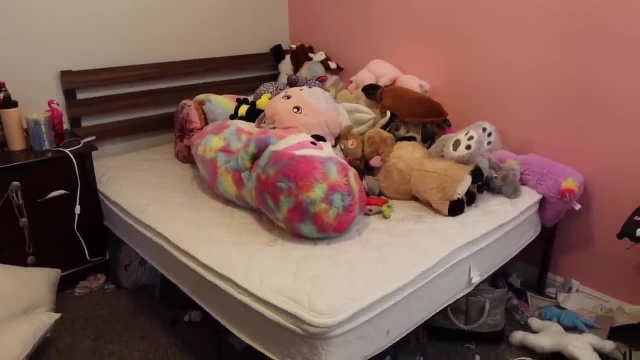 can see she's a stuffed animal lover and she is very attached to her stuffed animals, so I'm just gonna try to organize them a little bit better. I'm just gonna try to organize them a little bit better, but you know we're not going to be getting rid of any because she loves. 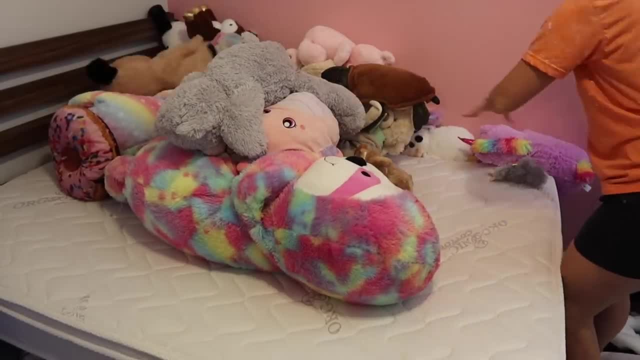 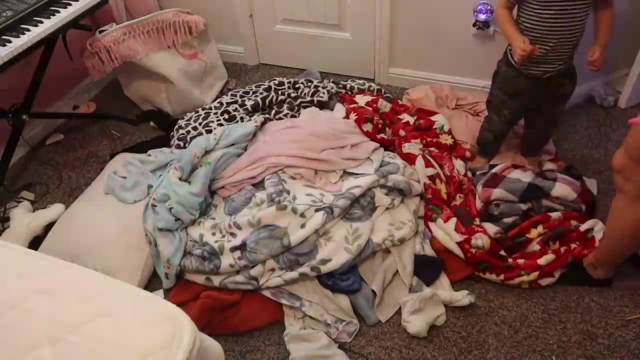 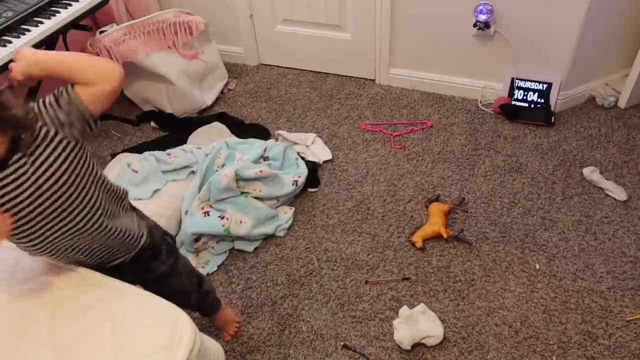 them so much. if you guys have an area of your house that you really don't enjoy cleaning, go ahead and put it on your to-do list. I promise when you get done you are gonna feel so proud of yourself and so satisfied. I dread doing Adrienne's room. 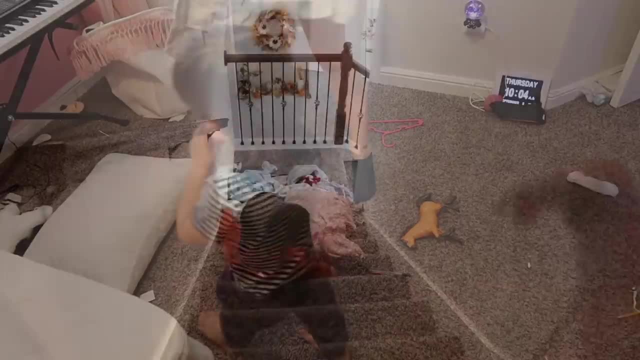 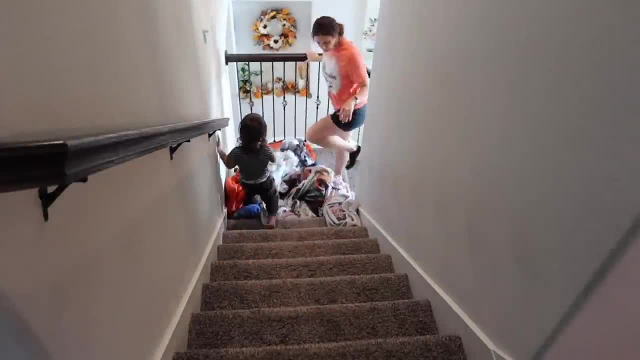 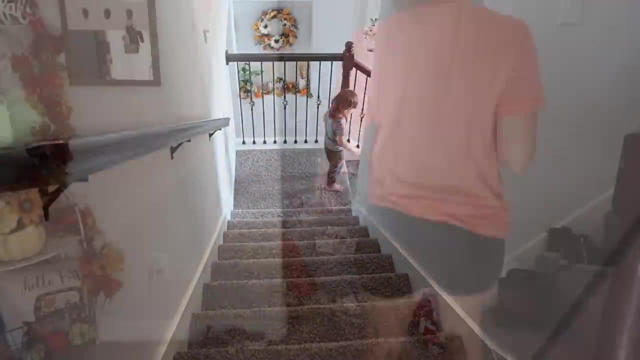 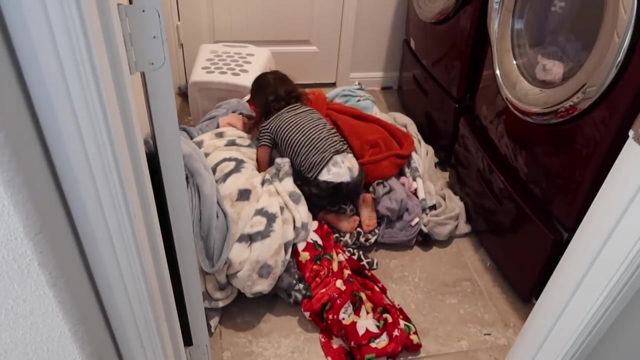 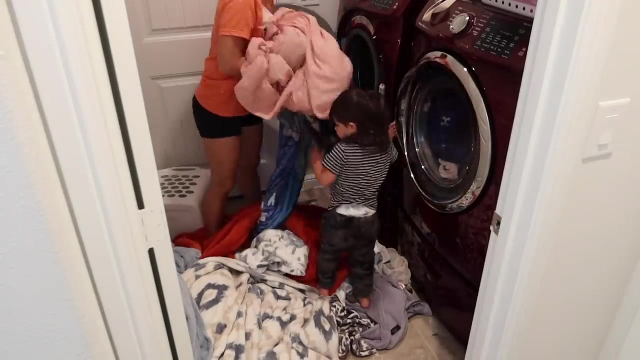 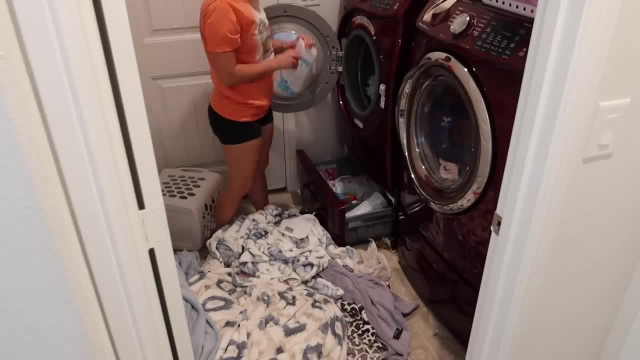 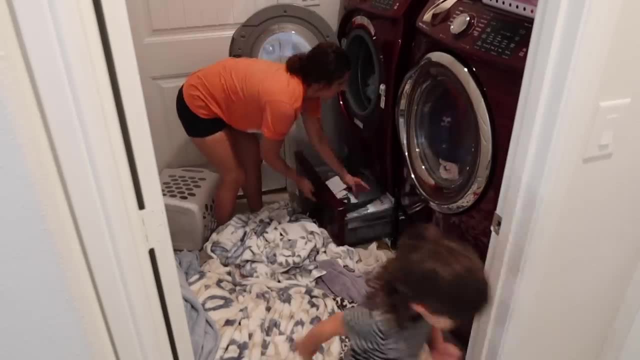 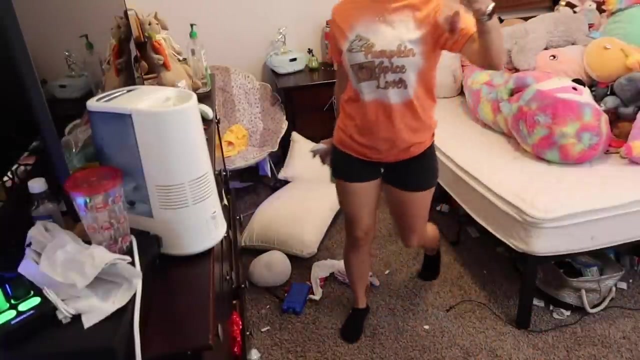 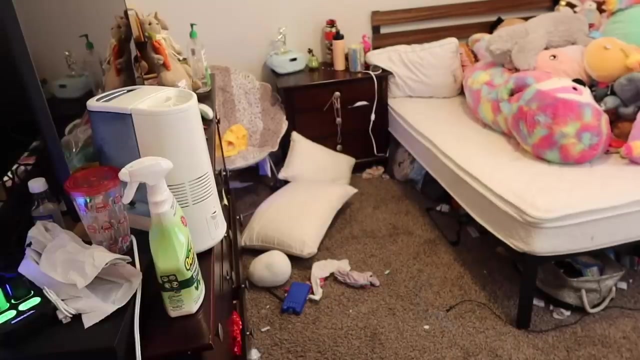 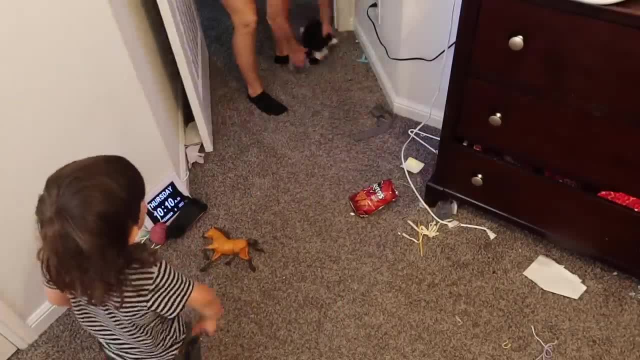 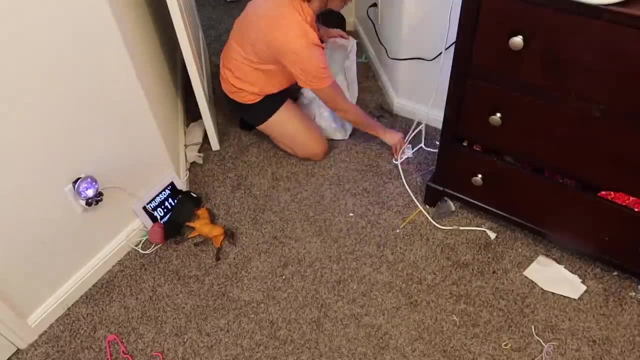 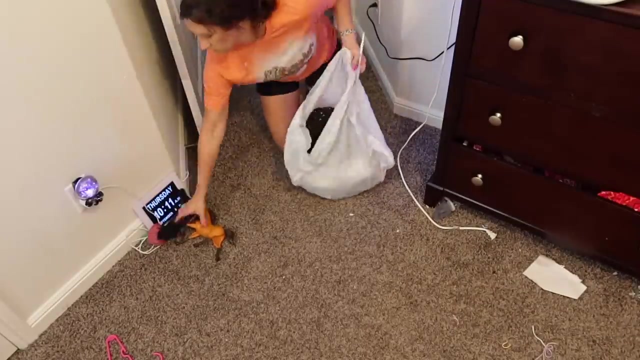 find in your kids' bedrooms. but I was not too pleased about it because, for one, I don't let my kids eat upstairs. I try to keep them downstairs. for one because I don't want the crumbs in the trash, And for two, we are a very managed and scheduled family. My kids only eat at certain. 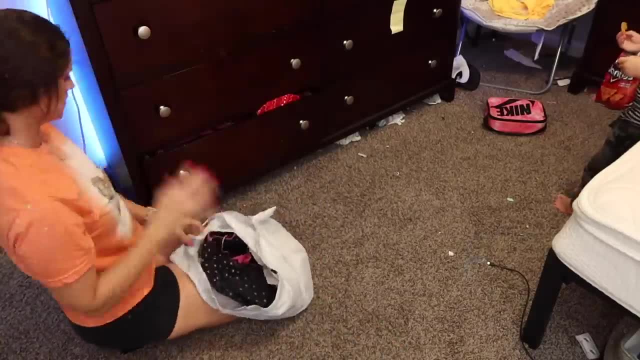 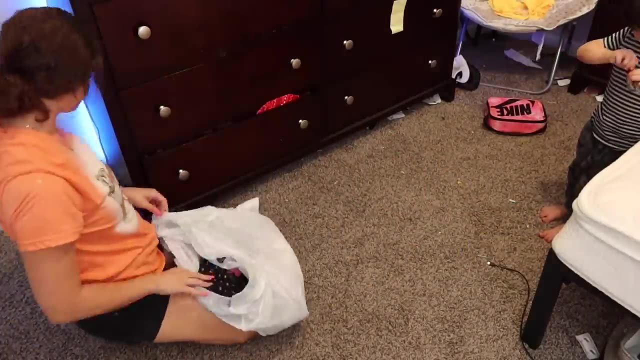 times and we only have snack time at certain times, So there really is no reason for them to be eating upstairs in their room. Let me know if you guys are the same way, If you have like a schedule for your kids on when they can snack and stuff, Of course, when they're little like. eighths age he snacks more often just because he's little. he's burning off tons of energy all day long. But as for my older kids, they mainly just want to eat out of boredom, and I do not let them do that, And that's always how it was done for me and my family when I was a child, mainly. 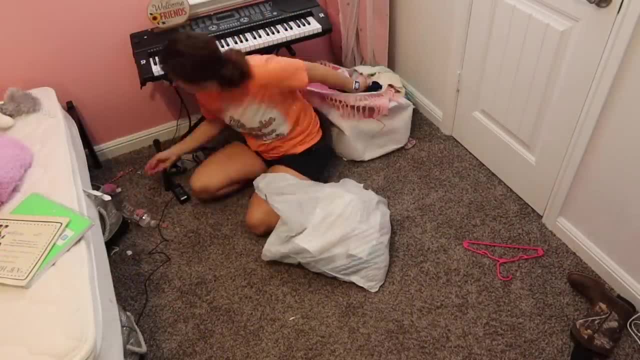 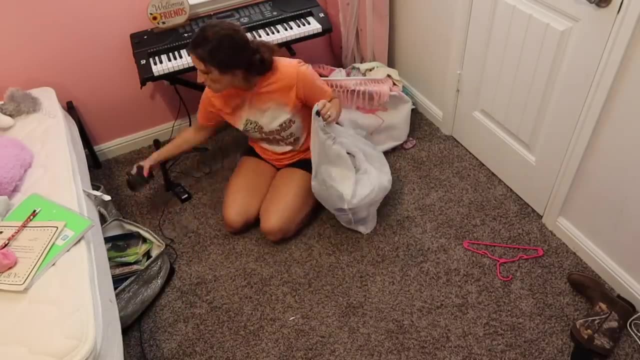 because there was five of us in the house and my carrot. my parents couldn't afford to buy endless snacks, So I don't know. I just implemented the same thing with my kids, which at first my husband was like what That's so weird? because his family 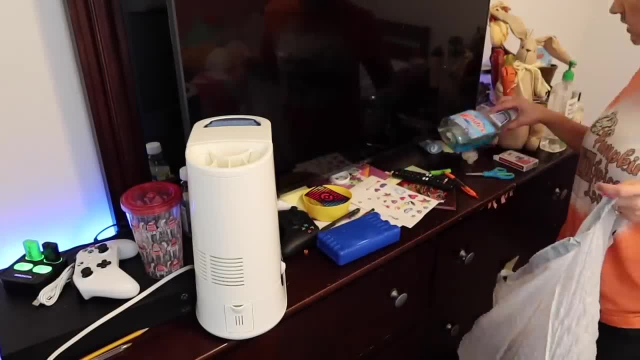 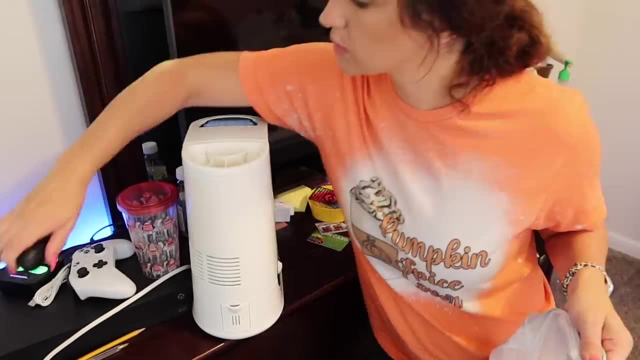 they could eat whenever they wanted to, as much as they wanted to, And for me that was just so strange. I'm like what? Like no, we can't do that, So I don't know. We just stuck with it. 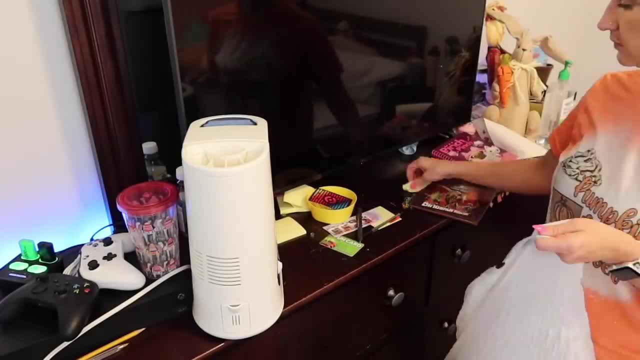 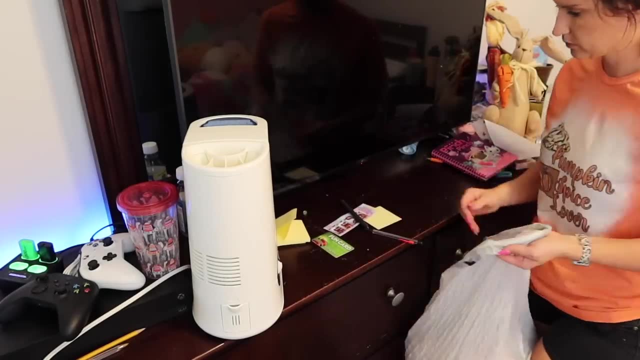 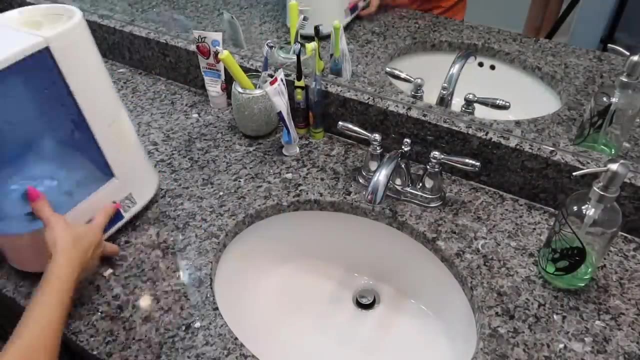 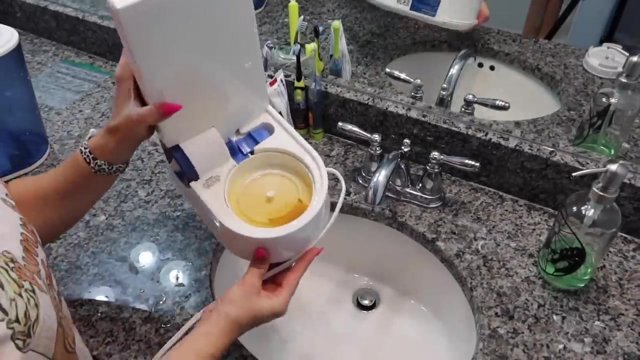 And plus, I think it's really important for kids to learn how to entertain themselves and not use food as a crutch Or like something to do just because they're bored. So, as you can see, Adrienne had the humidifier in her room and you guys, this thing was so. 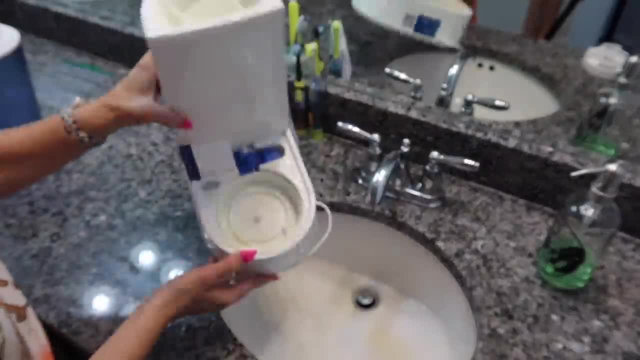 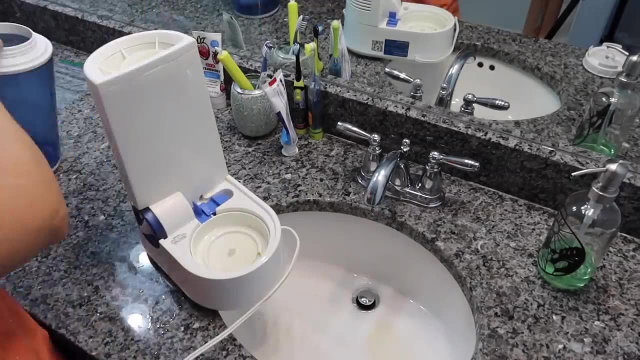 disgusting. It looked so nasty It was definitely time for me to clean it. So I'm going to rinse it out really well, make sure I get everything that's all gunked up in there out of it. The reason why she had this in her room was because 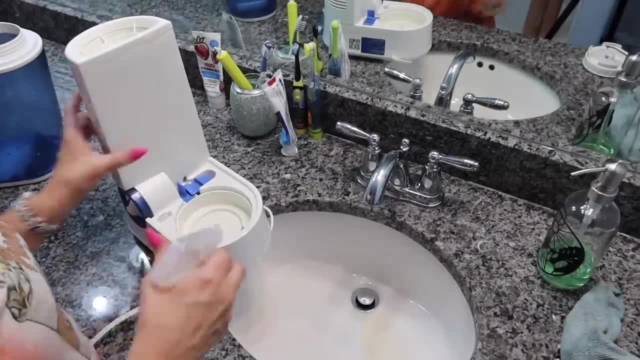 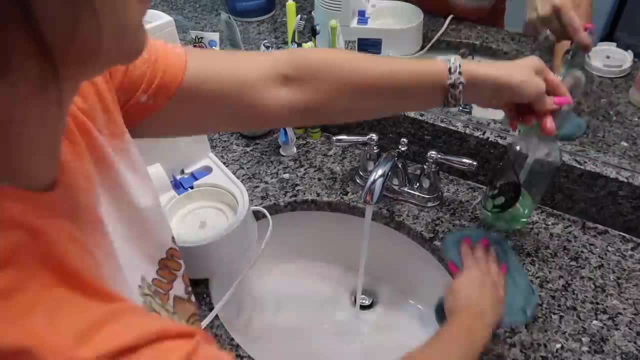 of course, at the beginning of the school year all the kids get sick and she just had like a stuffy nose that didn't seem to want to go away And it mainly bothered her at nighttime. So we use this plus put some of the like Vicks Rub stuff inside of it to help. 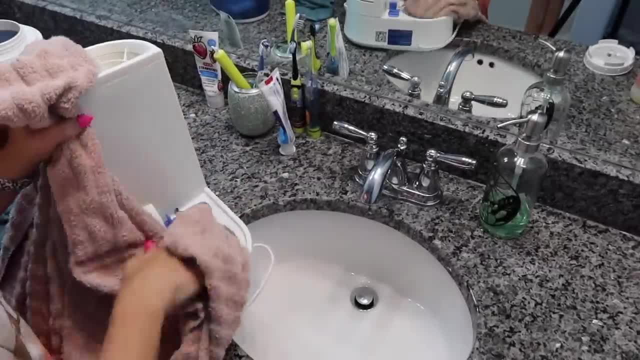 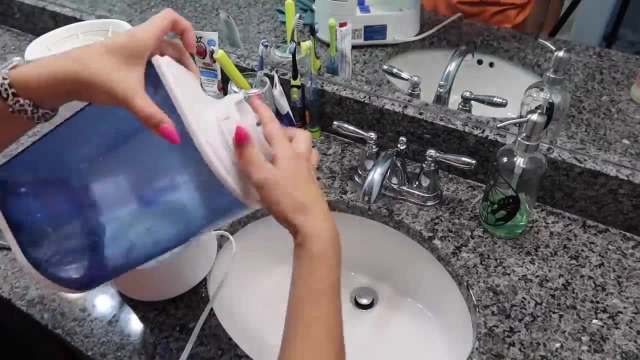 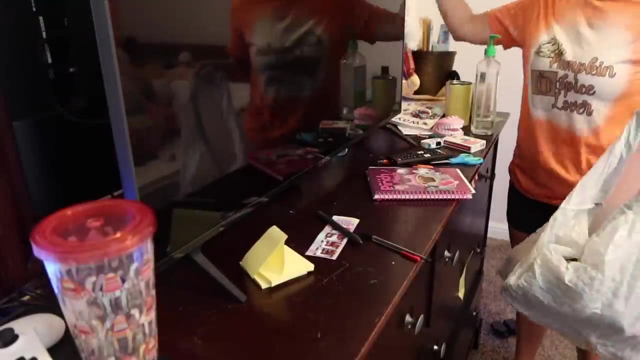 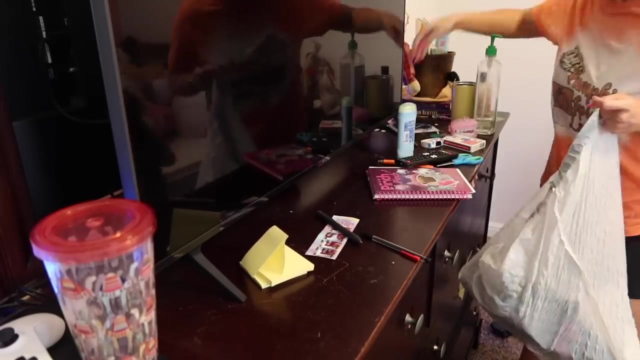 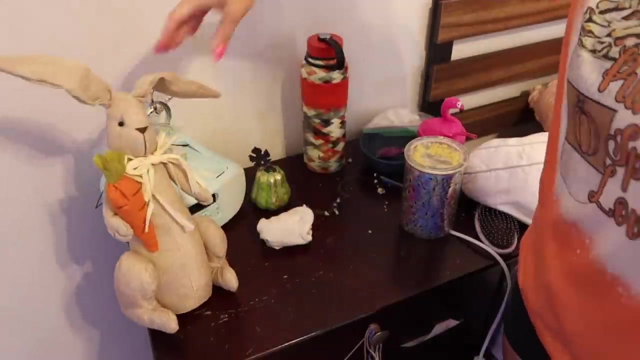 it just like make the whole room smell like menthol. So it really did seem to help her, but it was sitting in here for far too long. It was definitely time to get it out and get it cleaned up. When we made our trip to Virginia, my sister, Courtney, gave Adrienne this cute little scentsy. 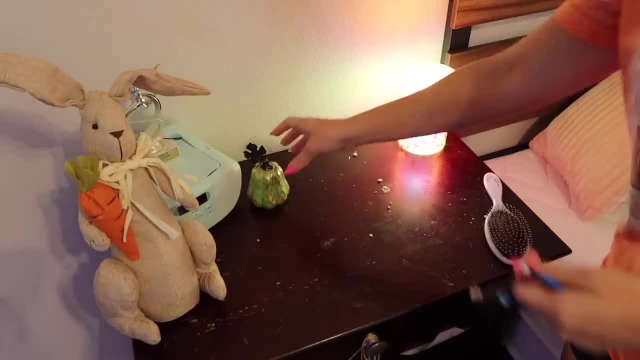 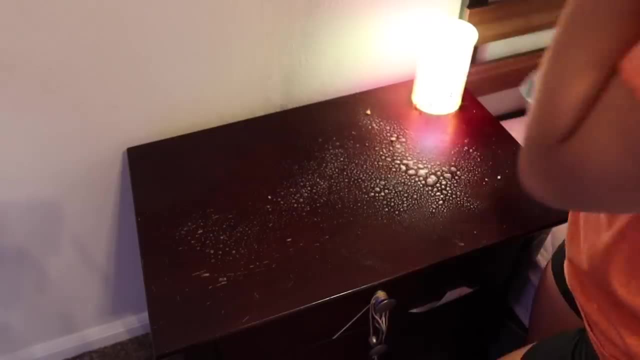 plugin thing right here And Adrienne has been loving having her own wax warmer in her room. but I could see that she was like digging and playing in the wax, So I told her. when she came home I was like, look, if I come up here and see this again, 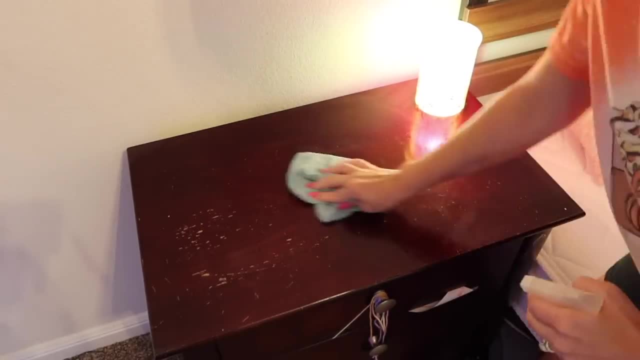 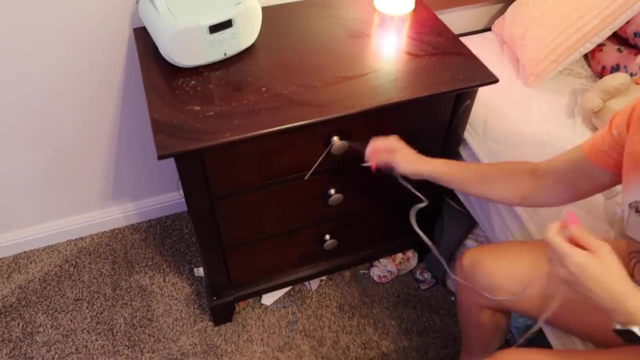 we will not have the wax warmer in your room because it was so disgusting, like just wax everywhere. I have no idea why she would even need to do that, So I just needed to turn it on, get it warmed up a little bit. 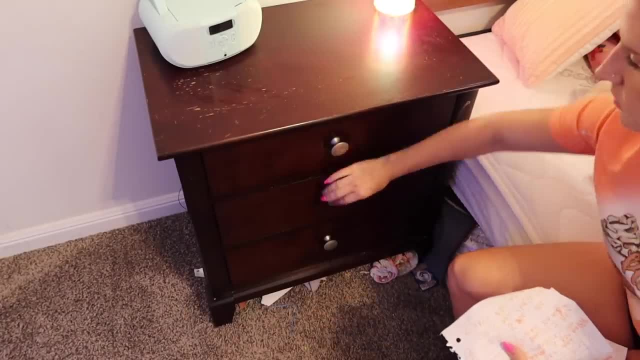 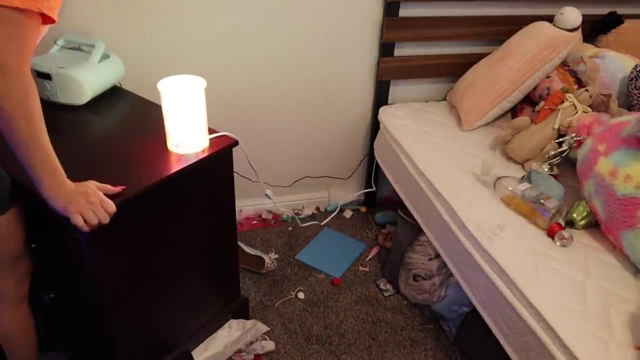 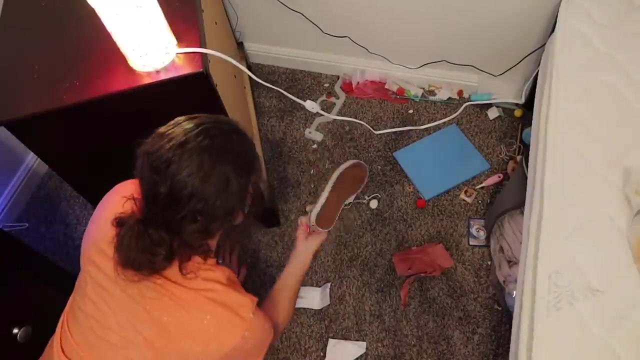 So I could wipe it out really good. So, as you can see, we had trash and clutter literally everywhere: under the dressers, under the bed, in the drawers. you're going to see, it was just everywhere. She loves like creating her own stuff. 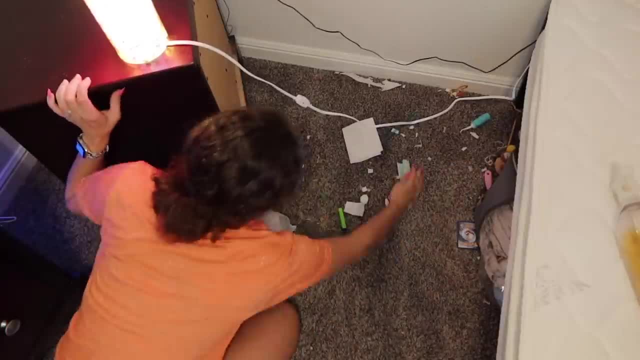 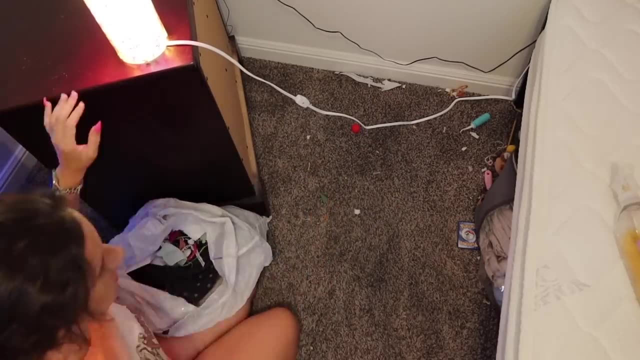 Like she makes her own slime. She uses her imagination and like cuts up pieces of paper and uses them for different things, But she's really bad about cleaning up after herself, as you can see. So I just wanted to make sure that I did a really good deep cleaning. 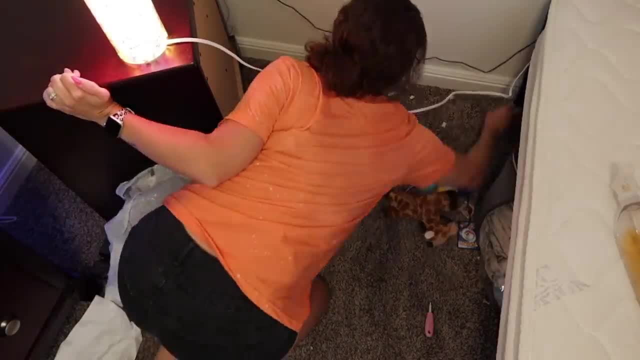 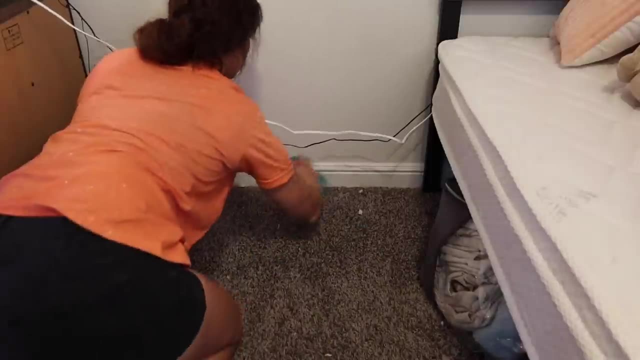 I do make her clean her rim, but of course you know, as a nine year old she cleans to her standards, which is basically shoving things underneath the dresser, underneath the bed. So I like to come in and do the deep cleaning every once in a while. 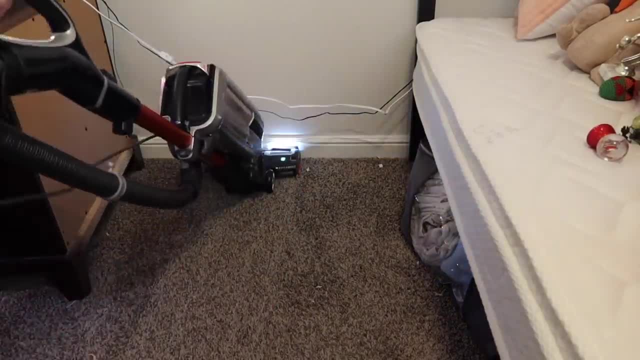 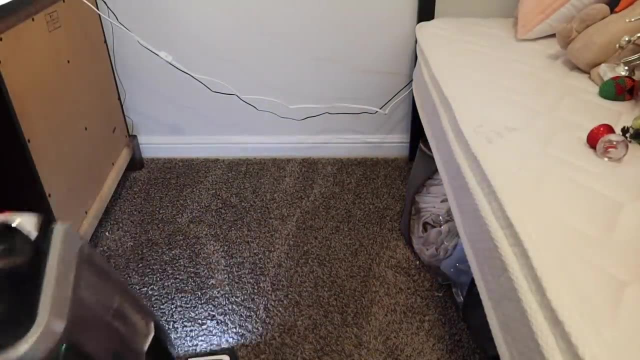 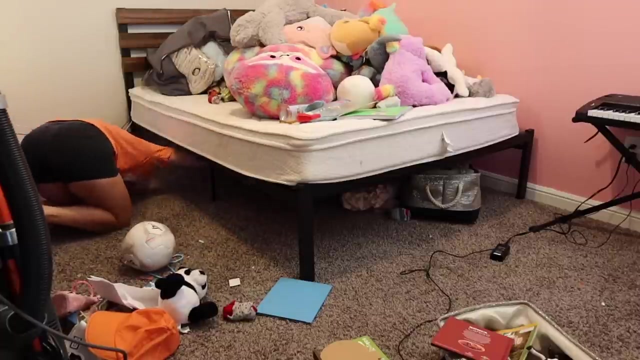 This is not too often, I'd say. I probably do this every couple months or so when I notice it's like getting out of hand And I really just want to give it that mother's touch. 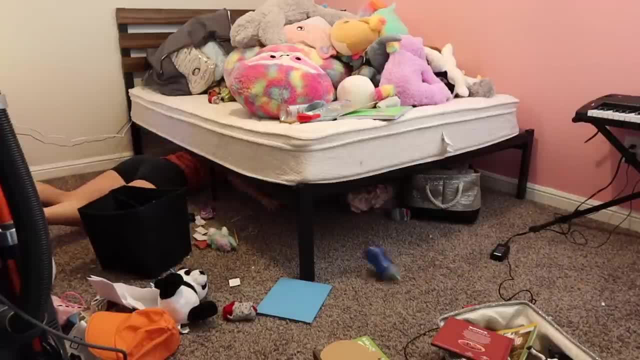 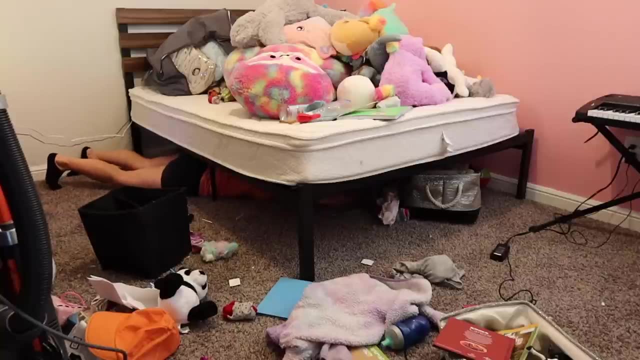 So I wanted to share something with you guys, since my videos are supposed to be motivational and hopefully help you in some way be more productive throughout your life- And I really do try to better myself. I love reading, and just learning. 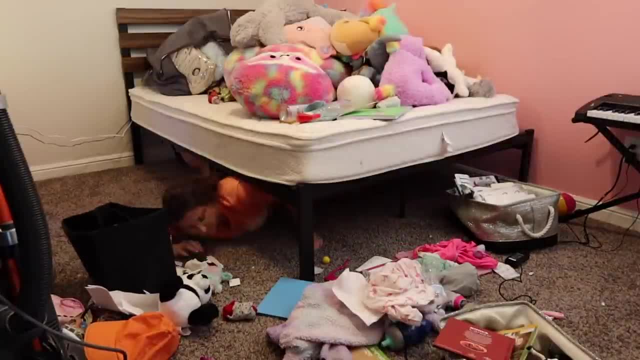 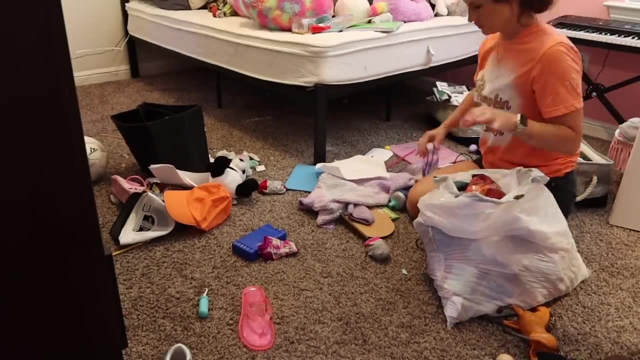 Like I feel like I am the lifelong learner. that's always the type of person that I've been, And recently I've been reading the book Atomic habits. I don't know if you guys have read that before, but It is an awesome book. 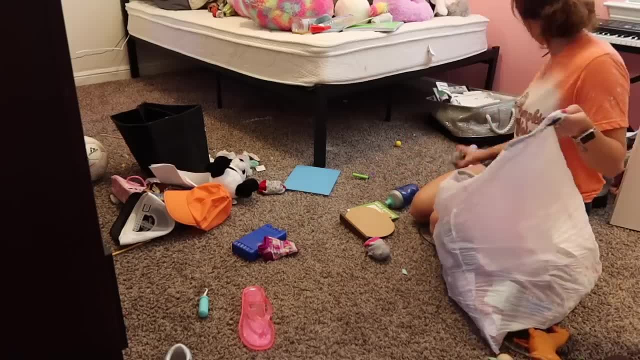 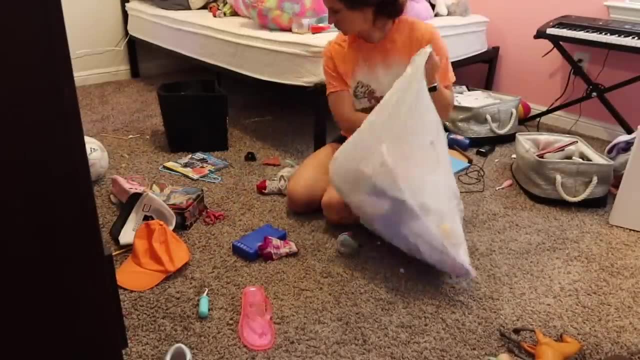 Definitely check it out if you are looking for something to read. but I wanted to share something with you guys that I thought was just very eye-opening and I don't know. it just made me feel like anything is possible, So I thought I would share it with you guys. 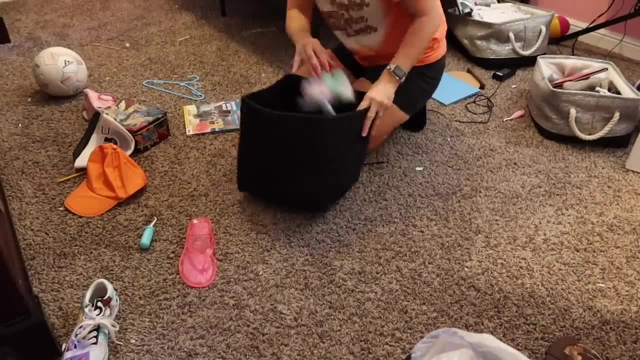 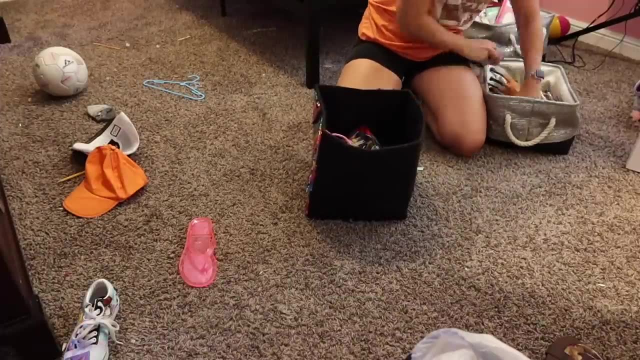 And basically, this book is about how to change your habits, to become a better person in whatever area of your life that you're trying to better, And one of the things that really stuck out to me was that he says you need to ask yourself. 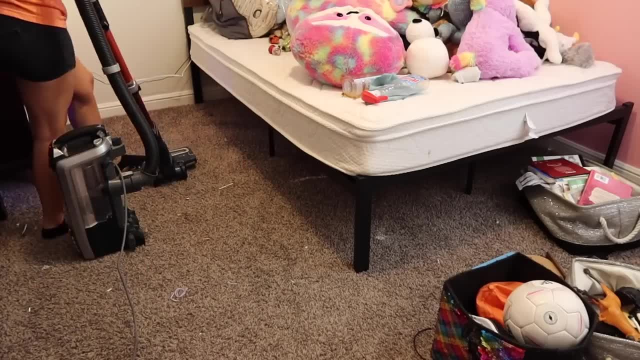 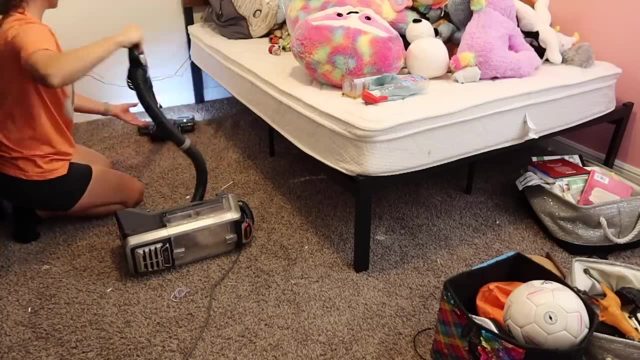 who do you wish to become? It's not necessarily the end goal, but it's the type of person that does those sort of things. So if you want to be a more organized person, you have to ask yourself: in a situation you know, what would a person who was organized do? 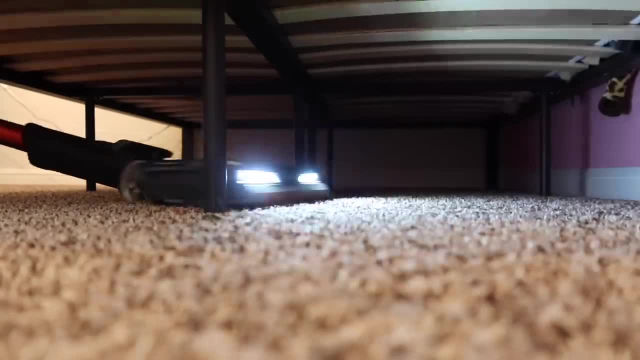 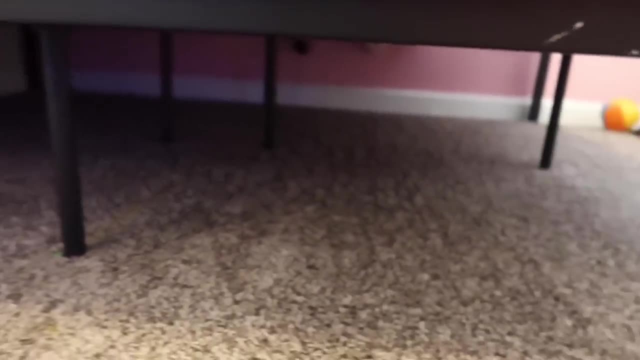 Like, would they just leave the mess in front of them how it is until they're feeling motivated, or would they tackle it as soon as they see it? And I really love the way he worded it, because basically he's saying that we don't change. 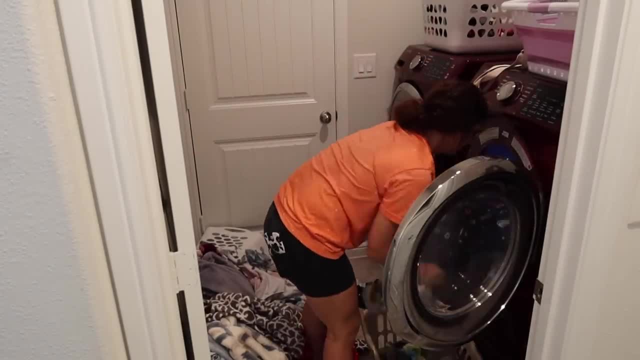 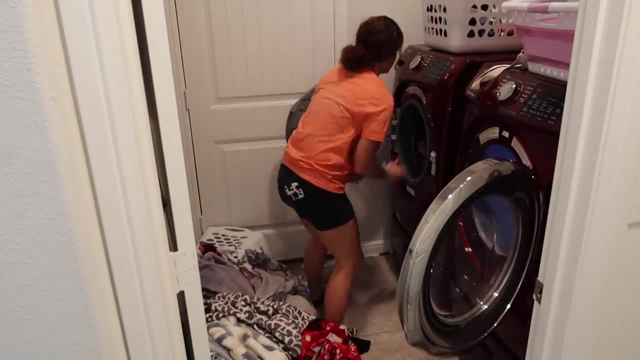 overnight. It is a gradual process. We change bit by bit, habit by habit, and every action that you take is a vote for the person you want to be. So, even if it's something small, if you keep doing it every day, it will add up and become. 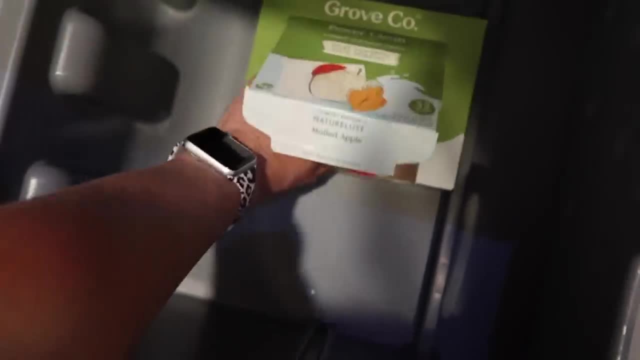 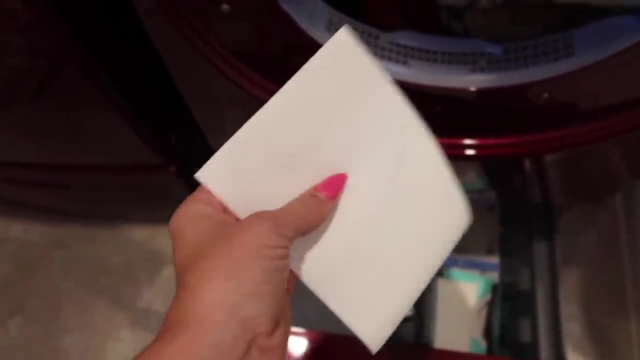 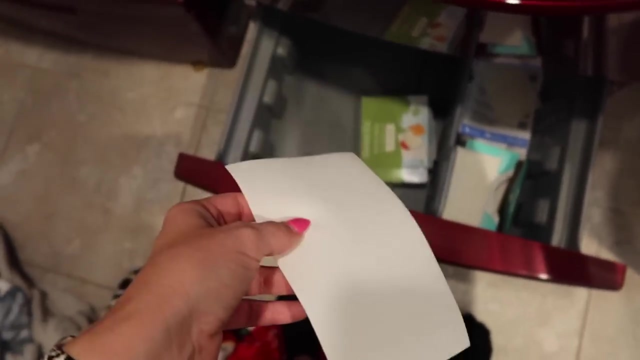 something so much more greater. You guys. these sheets are so cool. They almost feel like a Almost, like the true earth strips, like that material. It feels really cool. I'm really liking these a lot. It says they're dissolvable. 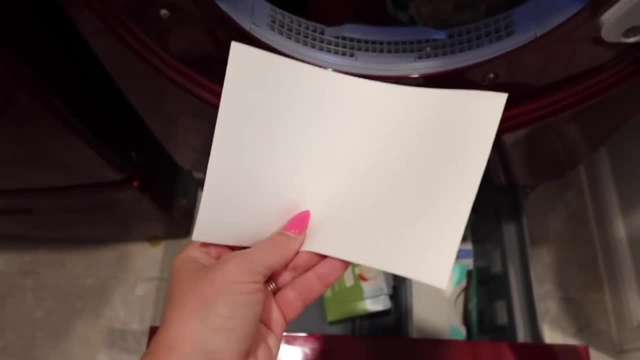 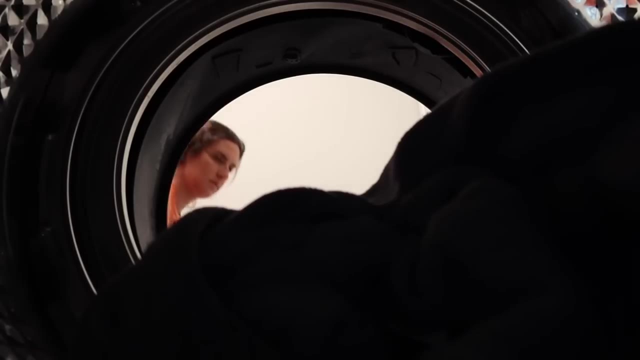 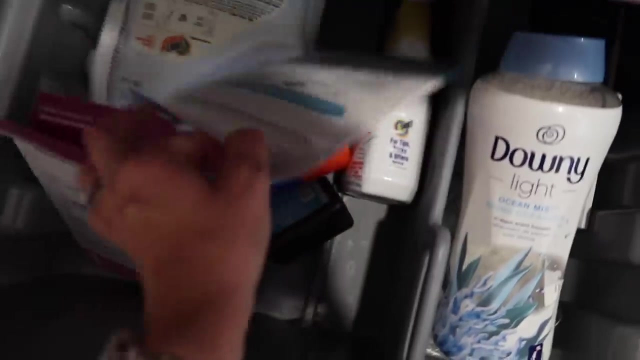 They don't really dissolve after a load of laundry, but I really like these so far. So, like I was saying, don't think that your efforts fall short or that they don't make a difference. They really do make those small changes every single day and before you know it you will. 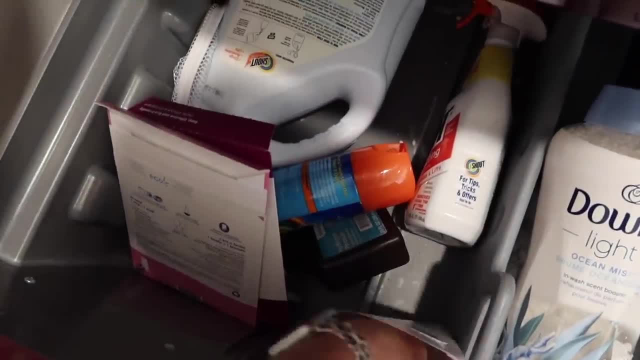 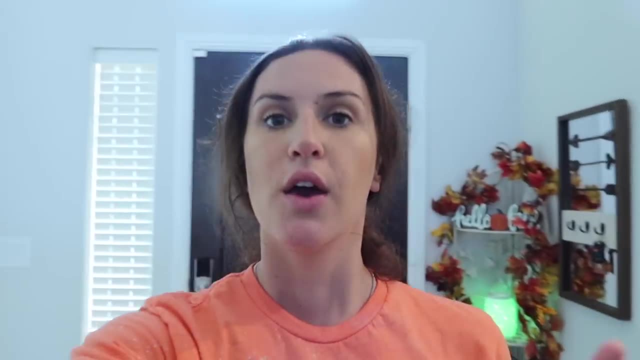 be the type of person that you want to be. You've always wanted to be organized, or whatever. it may be. All right, you guys. so I got more laundry going. I'm actually going to be taking a break from cleaning Adrienne's room and using my new 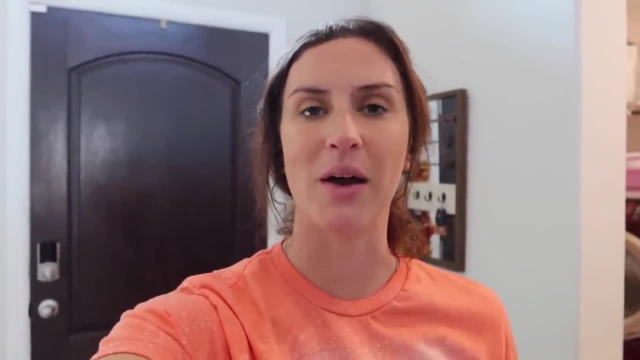 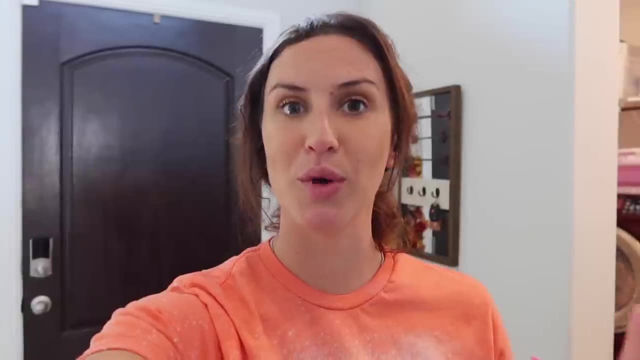 Peloton bike that I just got yesterday. I'm beyond excited about it. I want it to wait until it's nap time to use it, So right now is the perfect time. So I'm going to get back to her room after I do a quick cycle session. 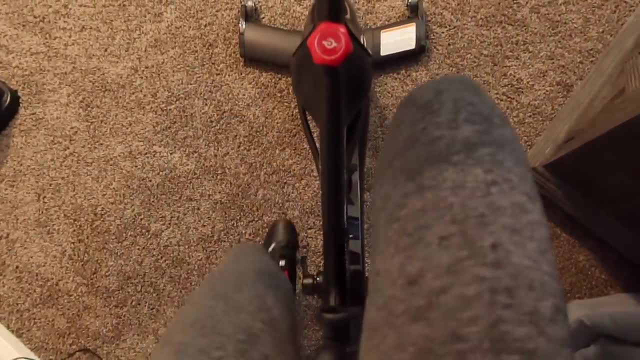 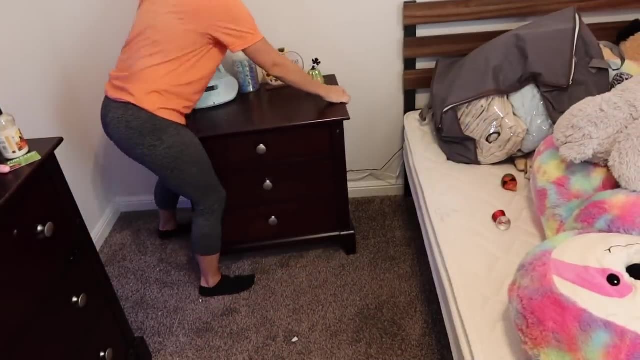 And it's just so funny That I decided to share this with you guys. I wanted to show you what I was doing in between cleaning and just have a little bit- I don't know better- insight of like how long it actually takes me to do these projects, because I feel 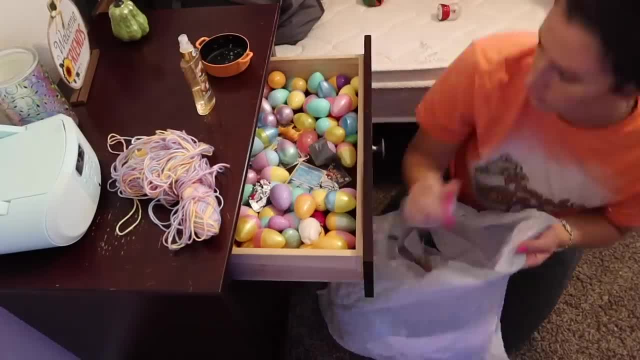 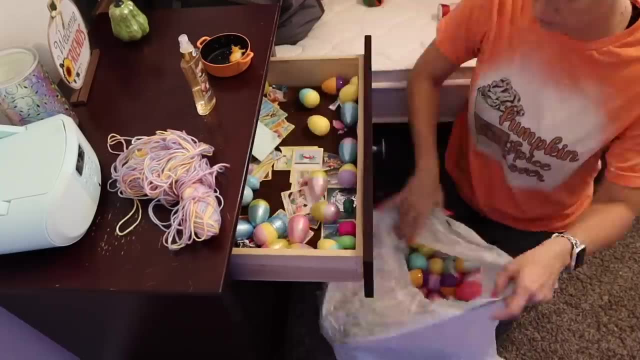 like. sometimes it seems like, you know, it doesn't take me that long, but they are so time consuming. But one of the big reasons why I ended up getting the Peloton was because I felt like I was putting my health on the back burner. 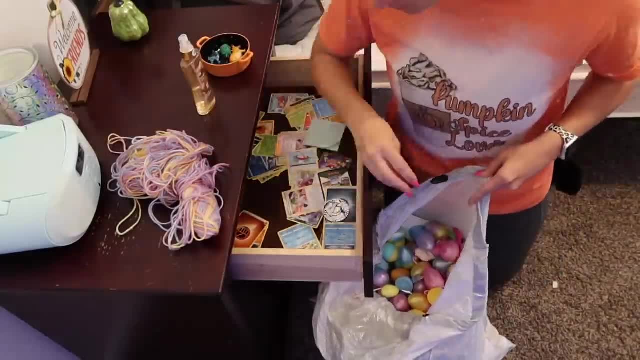 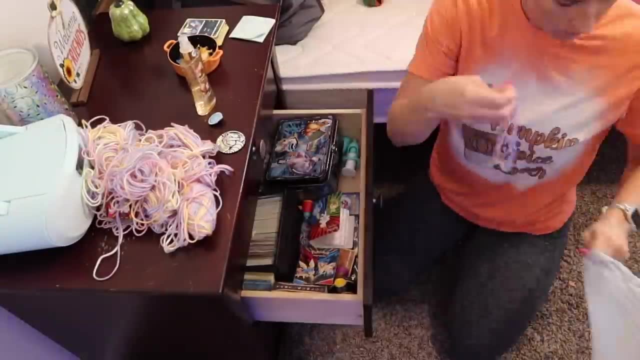 Like I wasn't eating as healthy as I used to. I wasn't eating as healthy as I used to. I wasn't working out nearly as often as I used to compare to, like before I started doing YouTube. and don't get me wrong, you guys, I love YouTube and I love what I do, but I 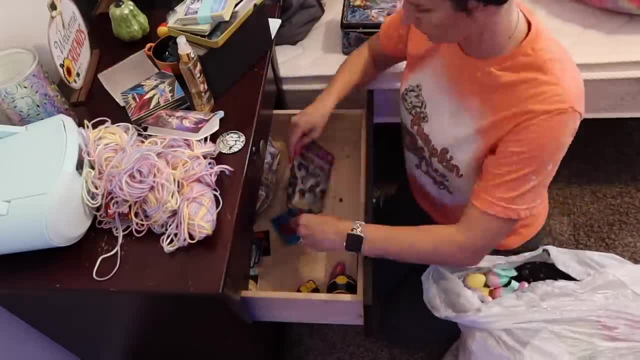 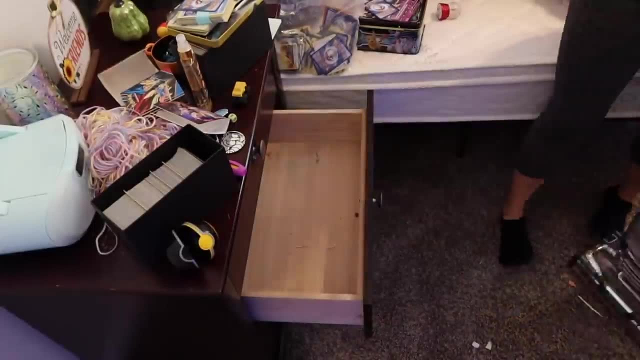 really was putting that before my health and my fitness, which has always been kind of number one for me. I've always considered myself a person who just really cared about health, and nutrition and like taking care of myself And I just wasn't doing that. 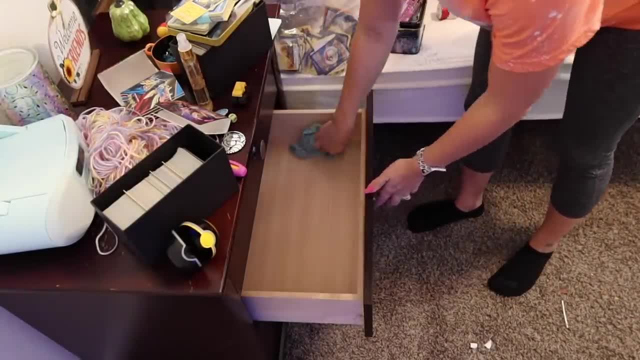 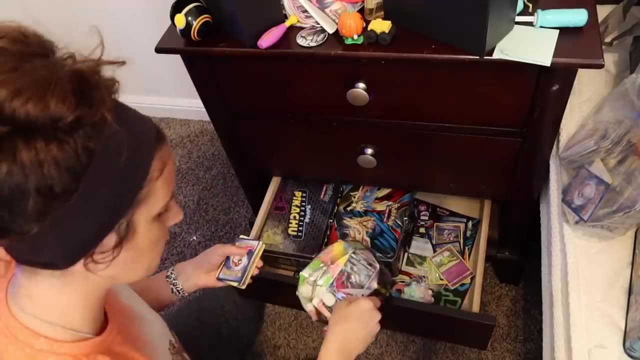 So getting this Peloton has been really exciting For me because I can stop whatever I'm doing, go get in a really quick workout and then get right back to it. So I'm just really excited about it And it kind of goes hand in hand of like what I was talking about, like whatever you want. 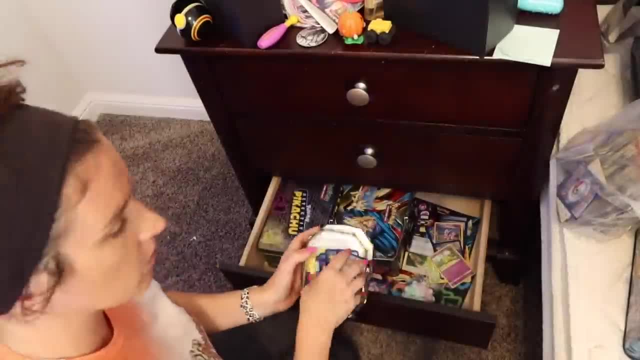 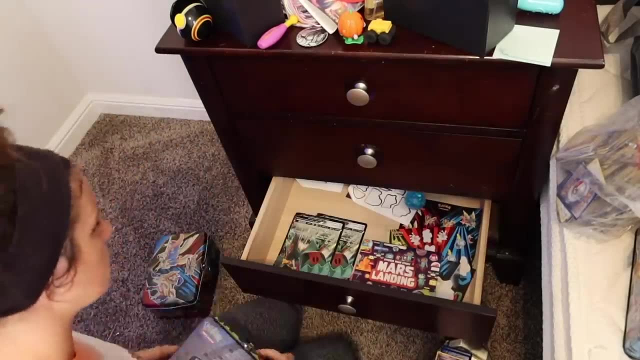 to change in your life, you have to take action, no matter how big or how small. it's just the gradual changes that you make every single day, And once you start doing them consistently, it will become a habit. And once it's a habit, you just do it unconsciously. 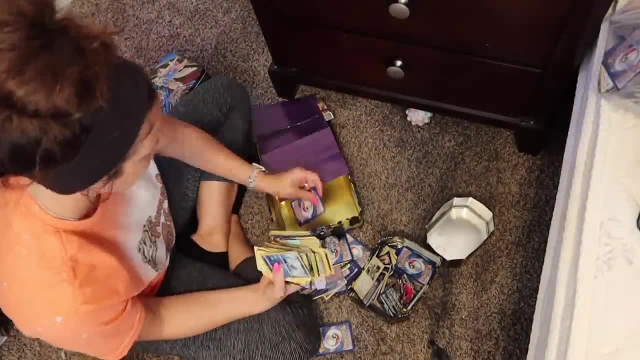 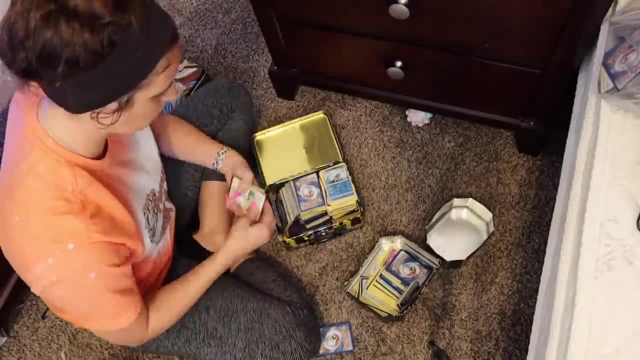 Like you do it Because you've just always done it and it's so much easier to do it, And so that's kind of how working out was for me, Like it was just something I've always did. I didn't have to think twice about but learning how to juggle, having basically a job like 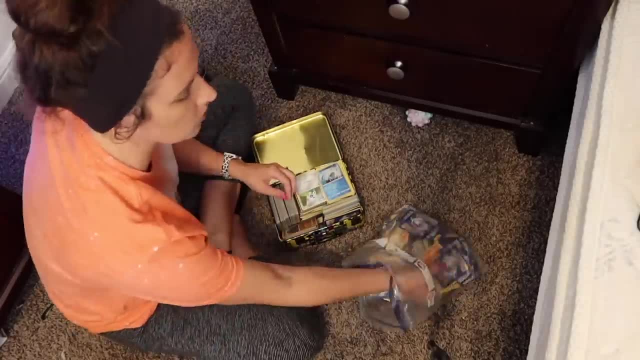 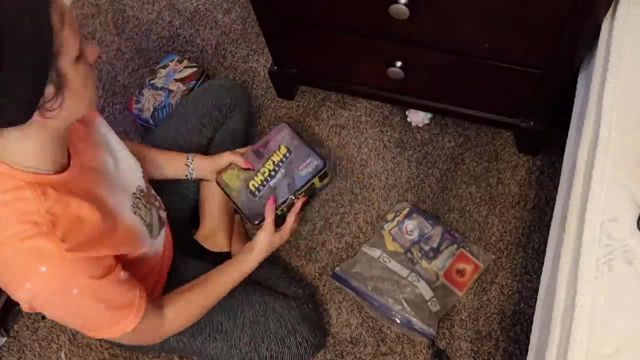 a work from home, job, as you know, my YouTube and trying to juggle my fitness. it was a struggle for me, So I am creating the new habit of trying to work out even if it's at home or if I can make it to the gym. 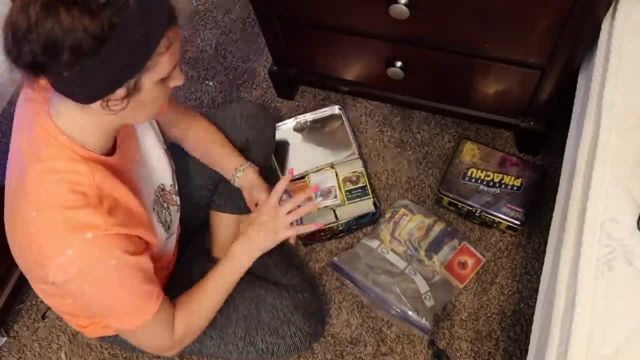 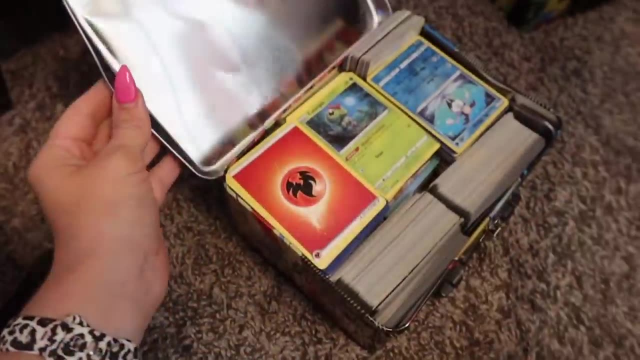 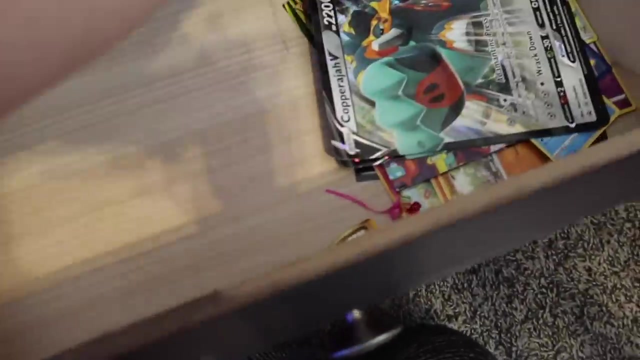 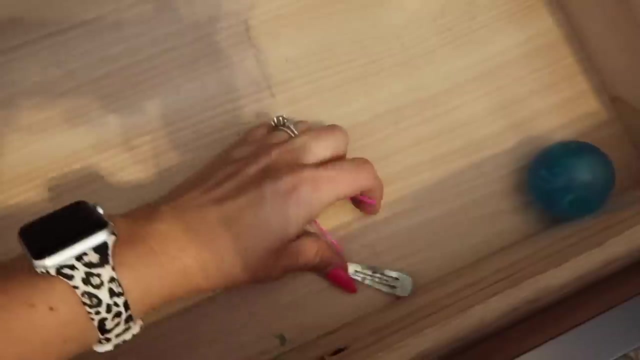 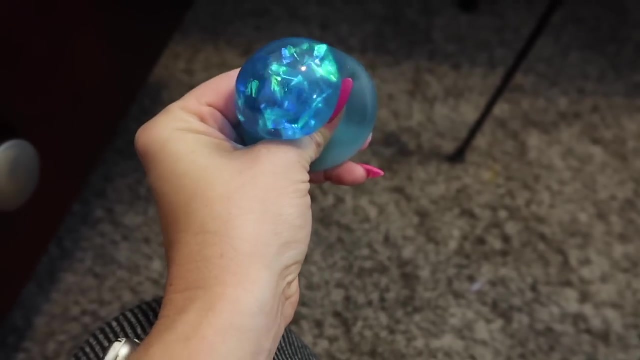 I'm definitely making the habit again of getting in my workout and taking care of my health. I'm sitting up in my lonely bed wondering what I just said to you. Anyone else love the kids like squishy balls. I think they're fun, but, as you can see, I've been decluttering her nightstand, which 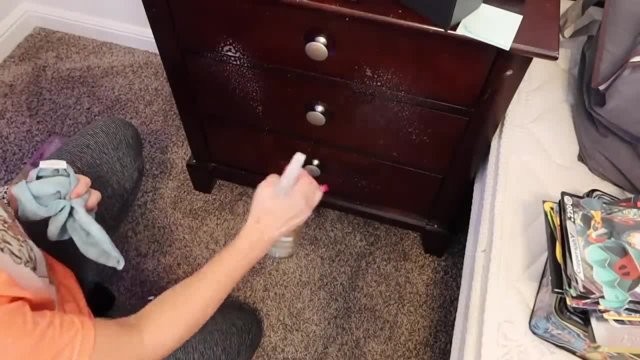 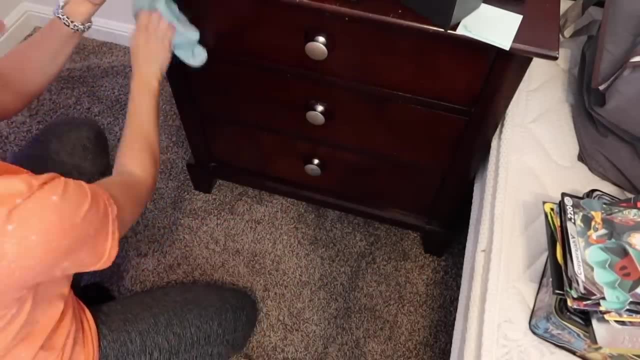 was full of not only toys but a million Pokemon. She loves Pokemon, As you can tell. she has tons of canisters of them, but they were kind of all over the place, So I really wanted to organize them again, put them in nice stacks, back into the canisters. 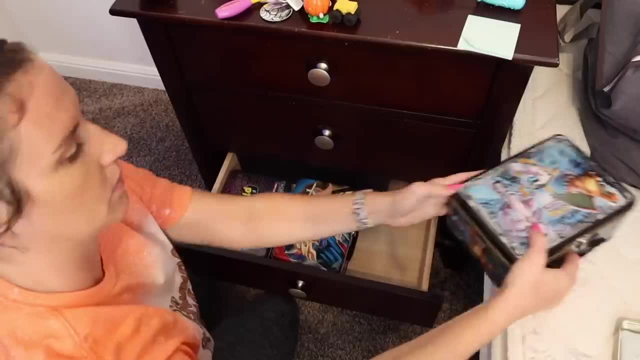 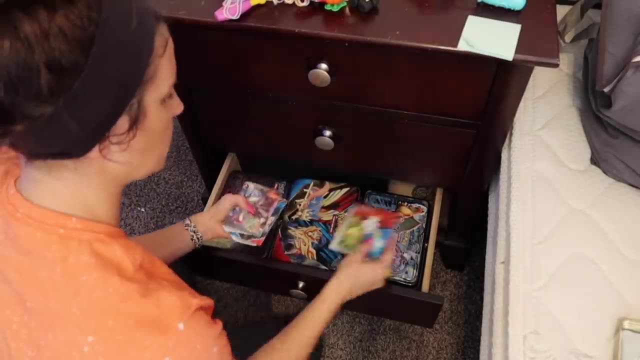 and neatly organized in here, because for one, I didn't want anything getting ahold of them and, you know, destroying them, Throwing them all over the house, So I was just trying to get them nice and neat for her. She also has some more in her big dresser that we're going to be collecting too, but 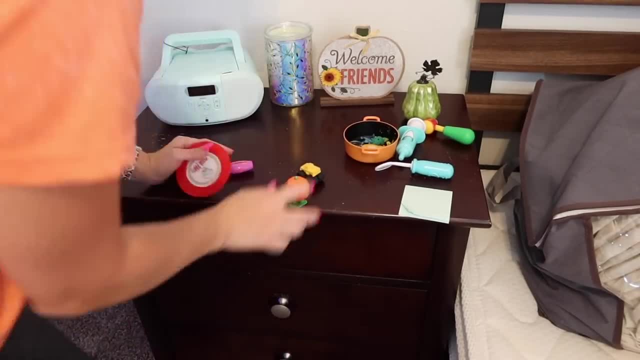 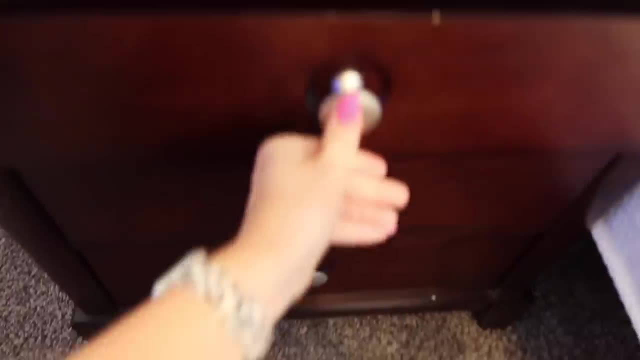 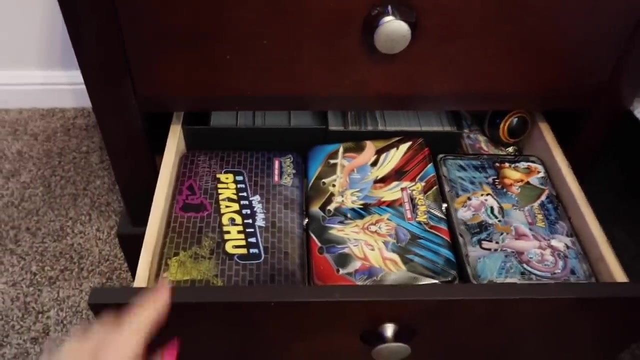 it made such a big difference. You guys, I'm like mind blown how organized and decluttered her room is when I get done. So now these drawers are empty and the bottom one has all of her Pokemon. nice and organized. I put these in the back just in case. 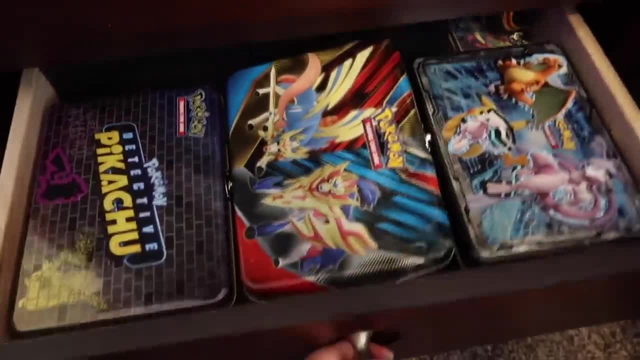 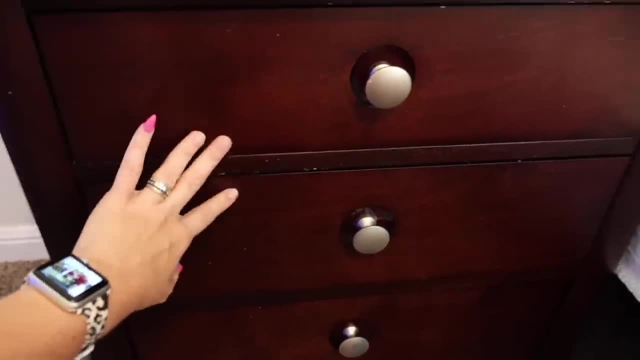 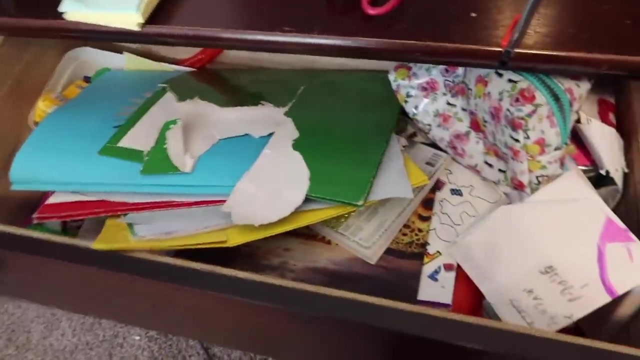 8th and open. She opens it up. I don't want him to pull everything out, so that works out great. Now she can figure out what she wants to put in these nice and neatly. So in these two top drawers she has tons of random stuff. 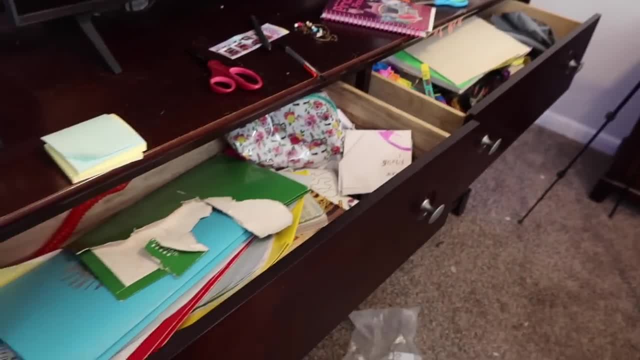 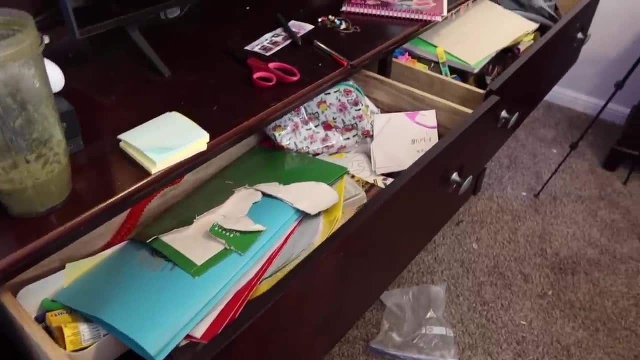 So I'm going to go through it, see what I know I can throw away. Obviously I don't want to throw away her stuff if I think it's something she's going to use or want to keep. So we're just going to see if we can make this look a bit more organized in here. 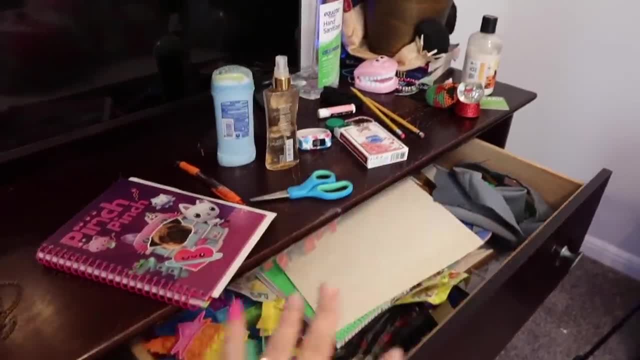 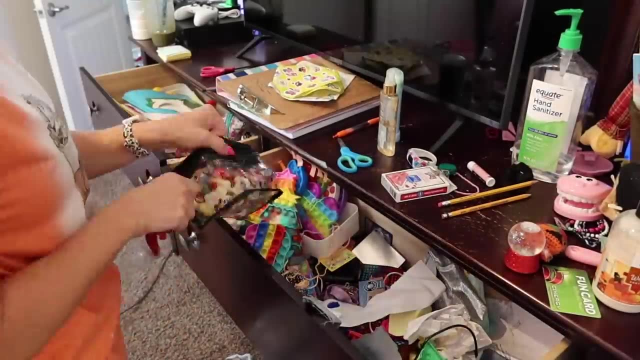 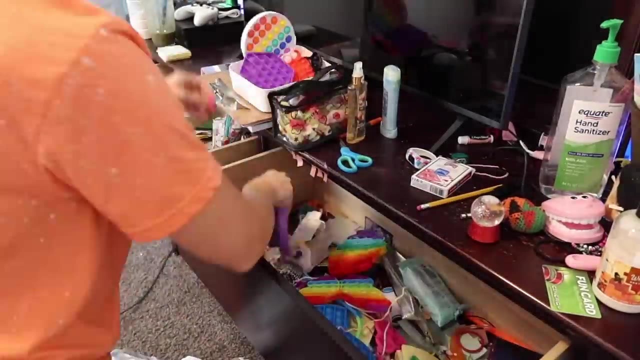 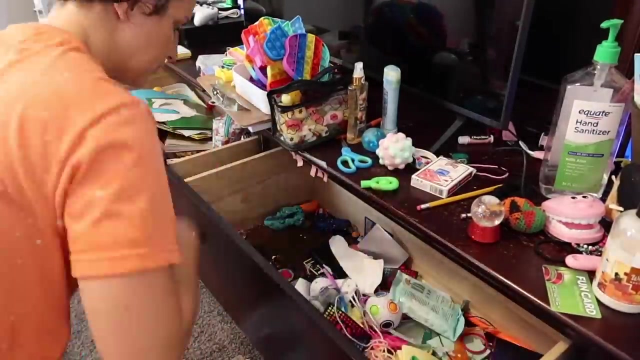 And then the few random things on top of her dresser- see if we can fit them in here possibly. I know you've heard it all before, but you are the love of my life. I knew when you came through the door that you are the love of my life. 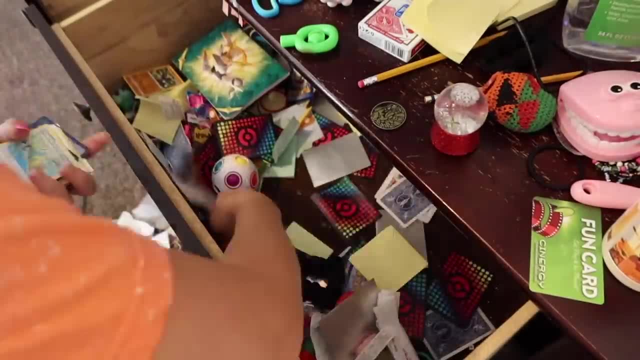 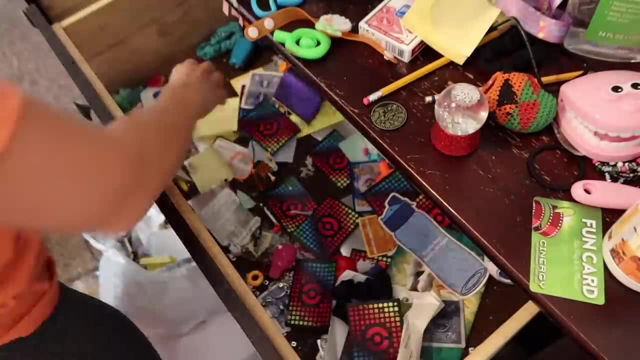 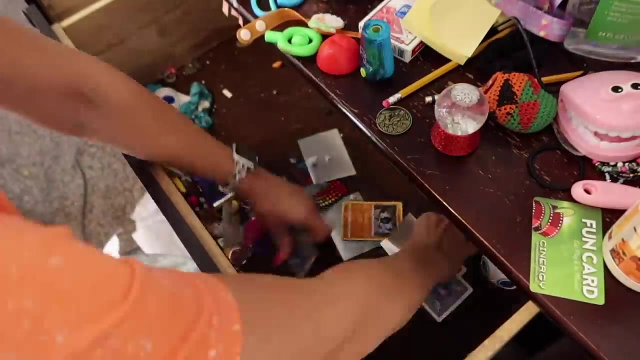 I could not believe the amount of trash I gathered out of these two dresser drawers. It was insane. I ended up filling up that entire trash bag. So much trash. Nothing's hard, everything is easy. with you around, No bombards, everything's easy. 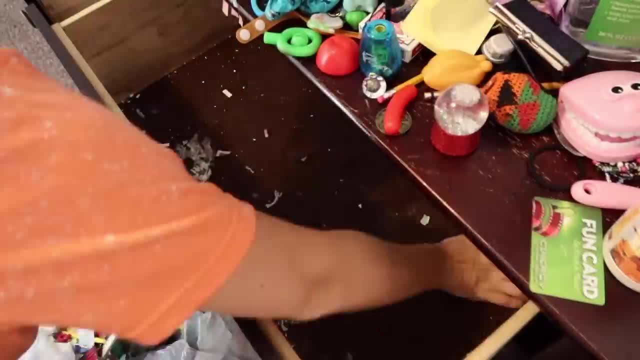 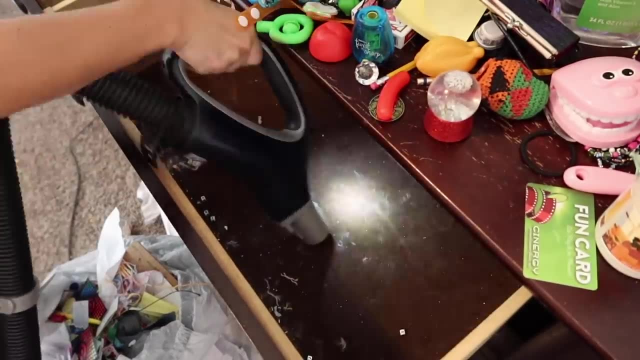 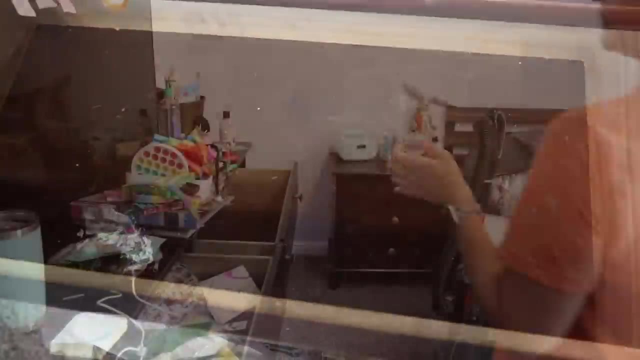 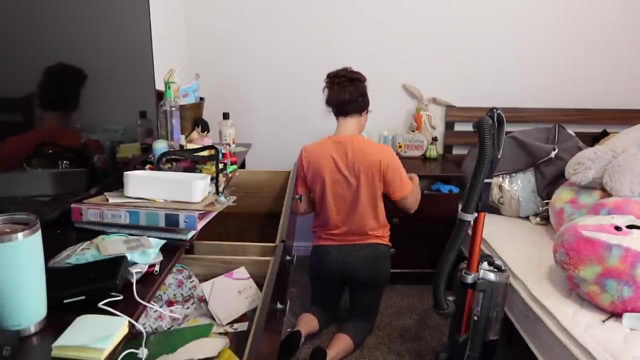 I'm so happy. No bombards, everything is easy when you come around. That's a stain of something, but it's all vacuumed. Can't really tell, but I vacuumed it out. I remember meeting you in a dream, thinking that's the love of my life. 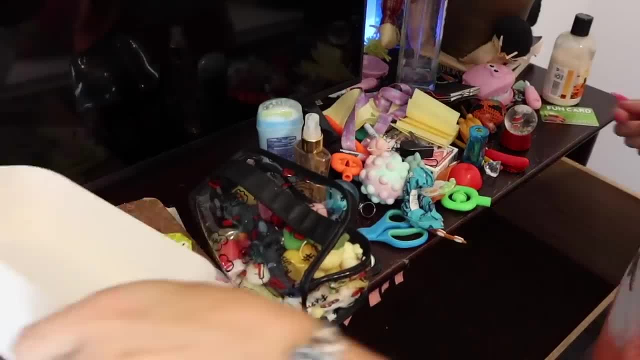 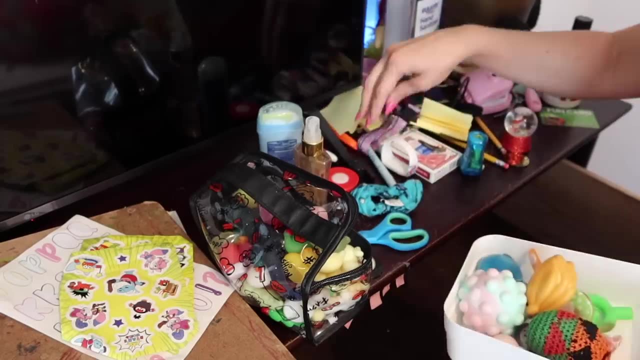 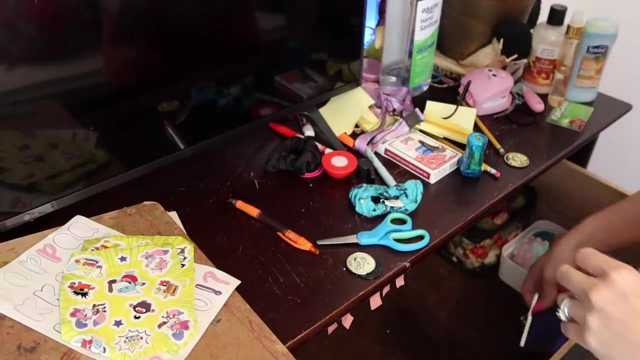 Most handsome man I'd ever seen. Most handsome man I'd ever seen. Most handsome man I'd ever seen. I said you must be. I believe I mentioned this already, but Adrienne is nine years old and her favorite thing, probably for the last couple of years now, have been the fidgets, the slime. 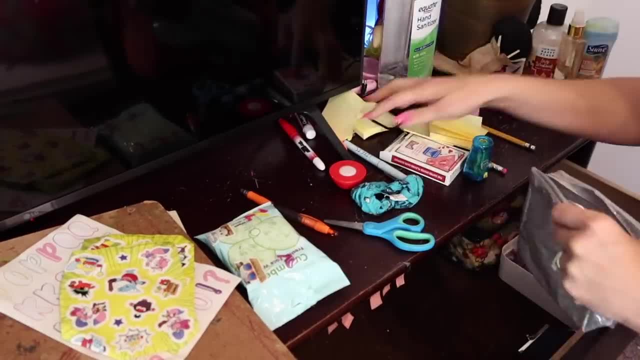 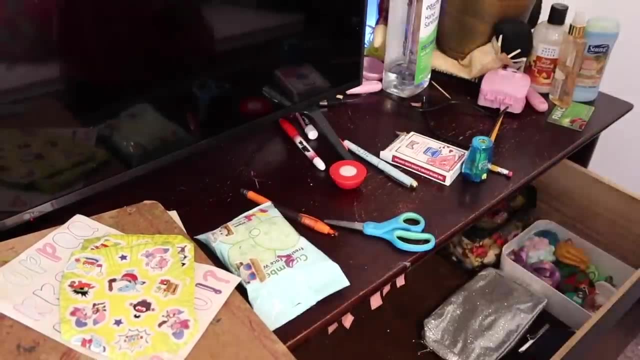 Like that's really all she plays with, and kind of same thing for my son. He is seven now and both of them they just love the fidgets and the slime. So we really don't have too many toys per se, Like she does love her stuffed animals, but toys wise. 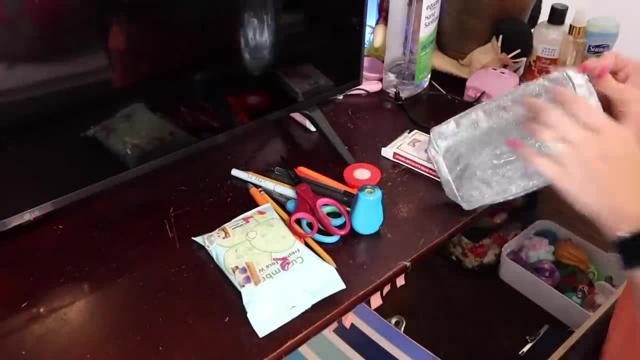 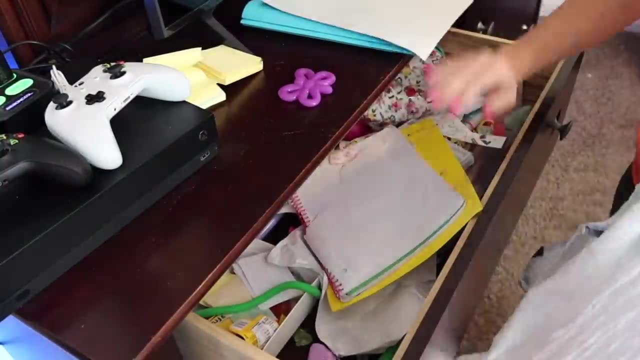 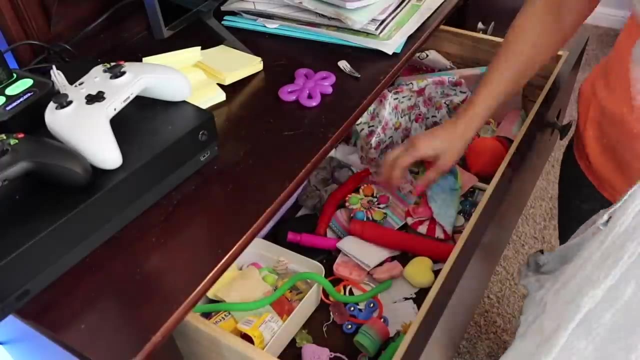 she really doesn't have too many. Thankfully, all of the things that she likes are like small, so I can organize them nice and neat into dresser drawers, but clearly I need to teach her the habit of keeping them organized after I get done decluttering and organizing them for her. 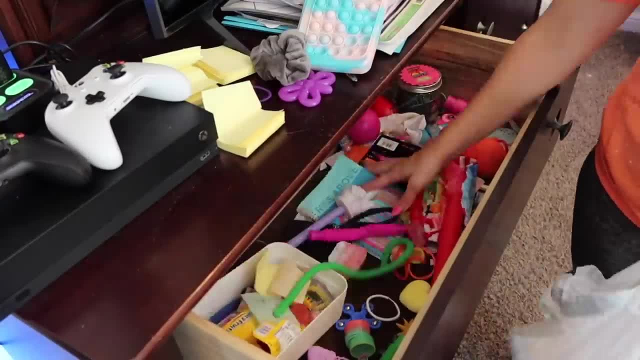 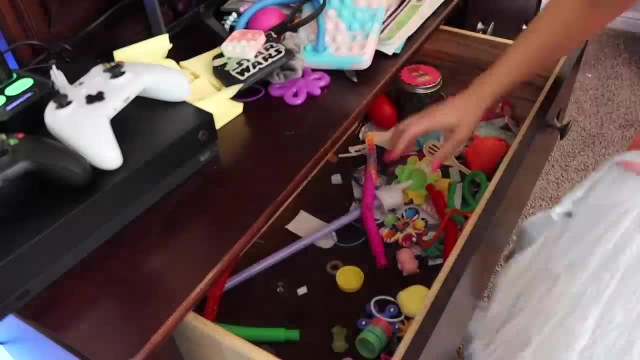 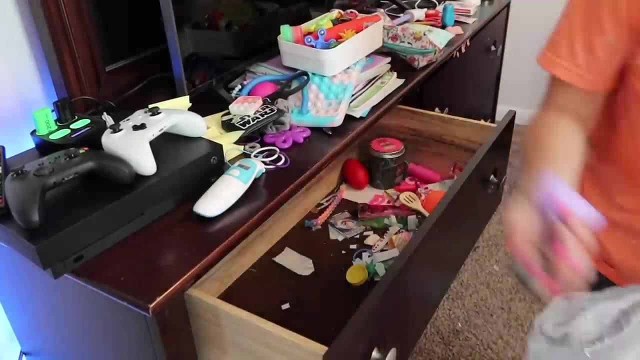 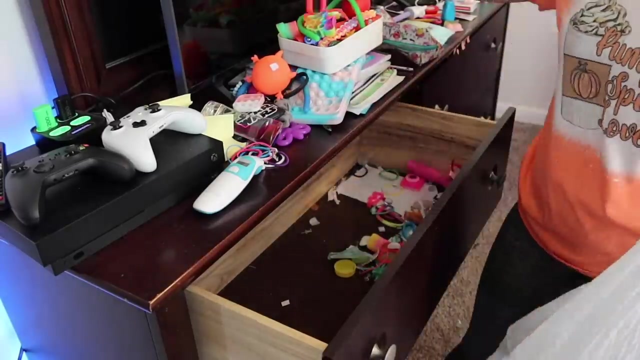 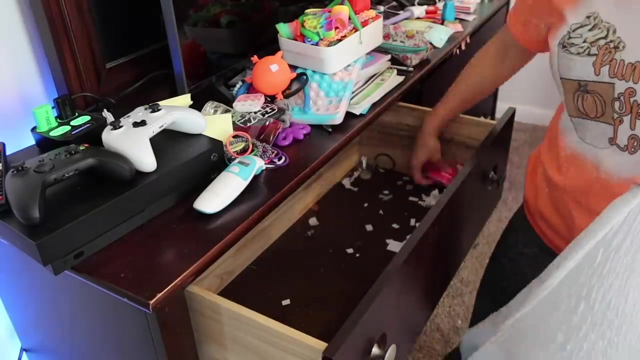 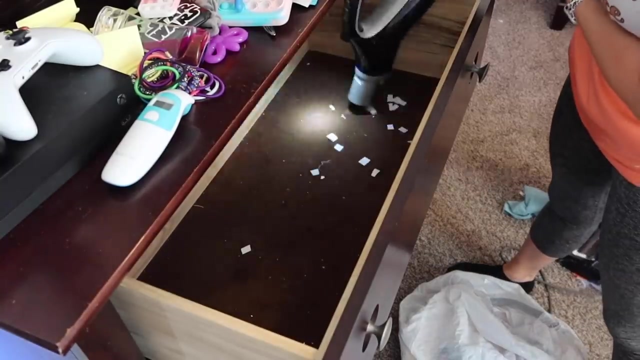 Don't let go of me, Don't let go, Don't let go. Nothing's hard, everything is easy with you around me, No bombas. everything is easy when you come around. Oh, Oh, Oh, Now Oh. 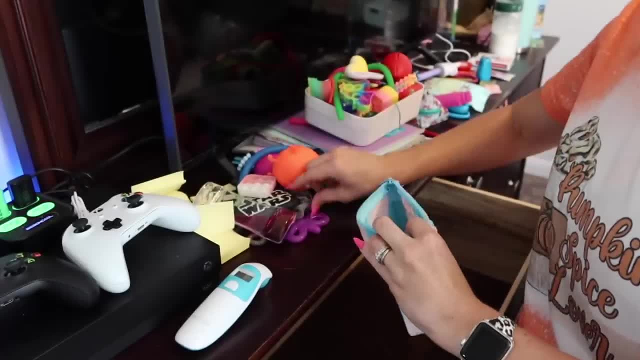 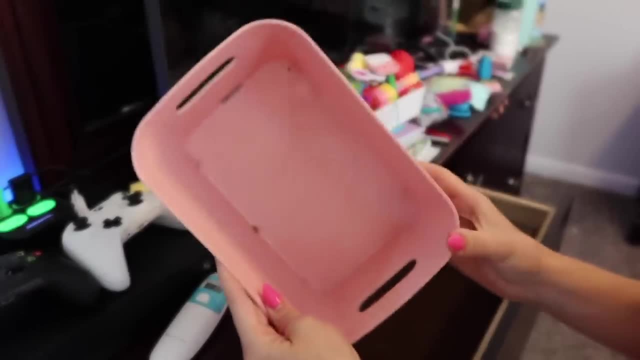 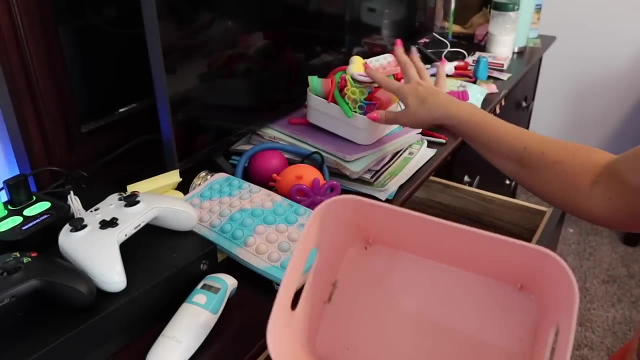 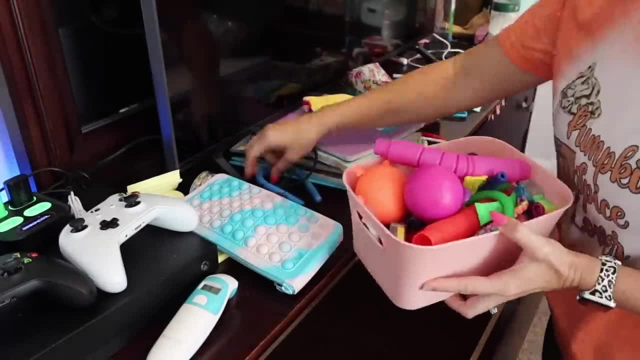 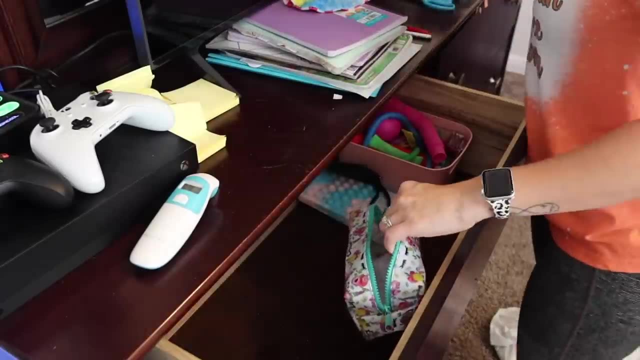 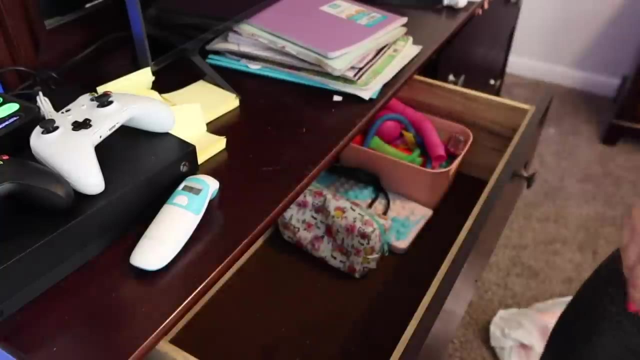 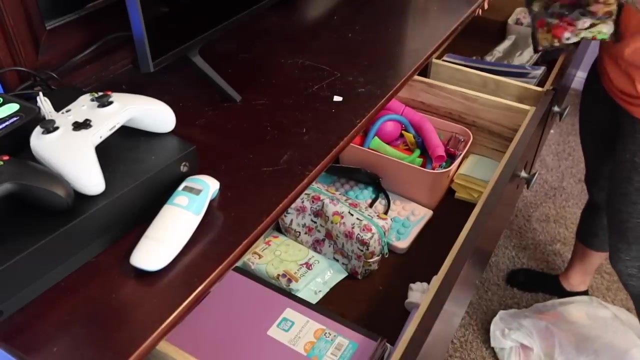 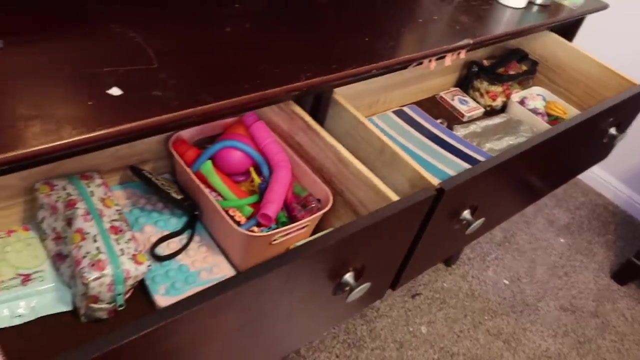 Oh, my goodness, you guys, these drawers, Look at that. Oh my goodness, Look at the transformation. So I have it a little bit more contained. We have her random books and stuff. I believe these are a lot of them are from last year. 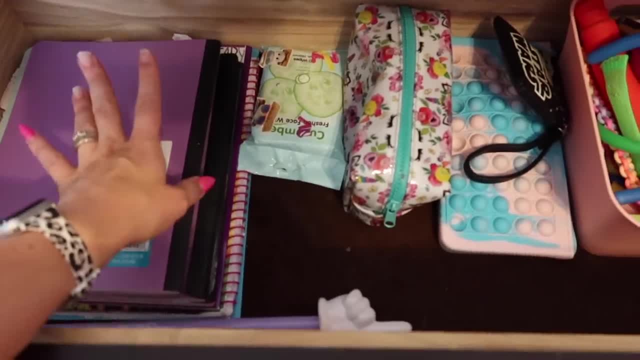 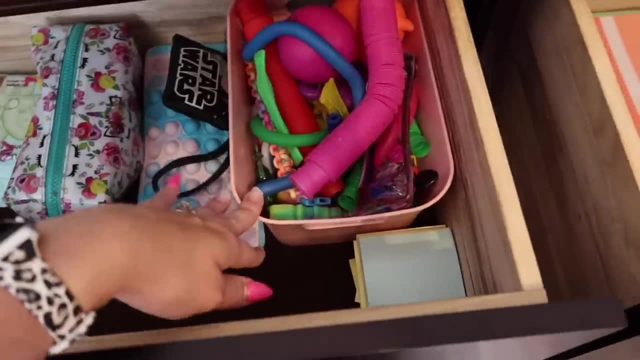 but I don't know if she wants to keep them for review, So we'll hold on to that. She has some little face wipes. I put all of her pencils and scissors in there: hair ties, fidgets, post-its, more notebooks and stuff. 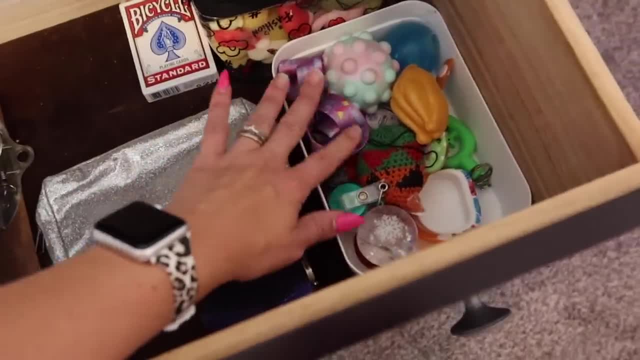 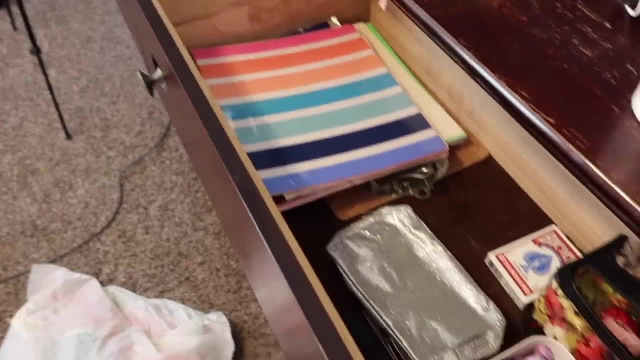 These are some more bracelets and necklaces, random little things and all of her mochis. So that is so much better. You can actually see inside the drawer now And, as you can see, I'm already on my second trash bag. 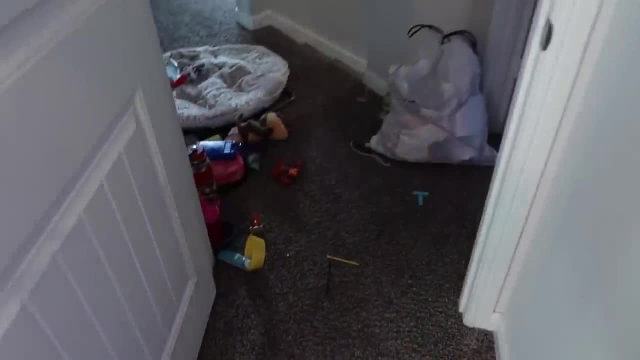 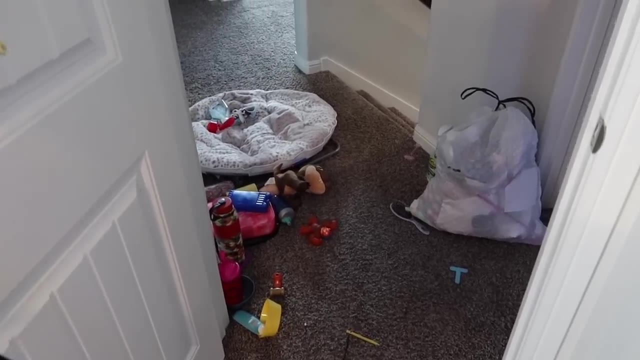 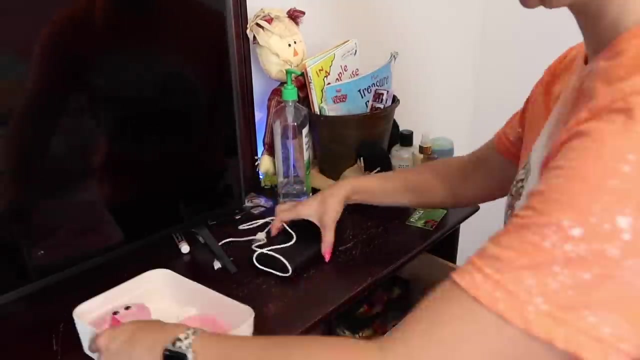 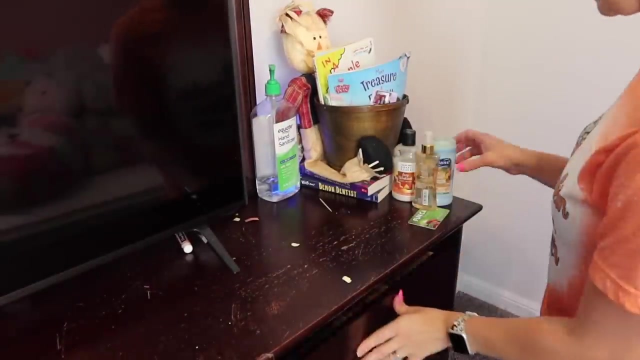 one full bag of trash already And I'm just kind of throwing out the stuff that either goes downstairs or into the boys' room while I finish sorting out her room. We are almost there. You can see right in the background. this is all of the stuff that we already have in the drawer. 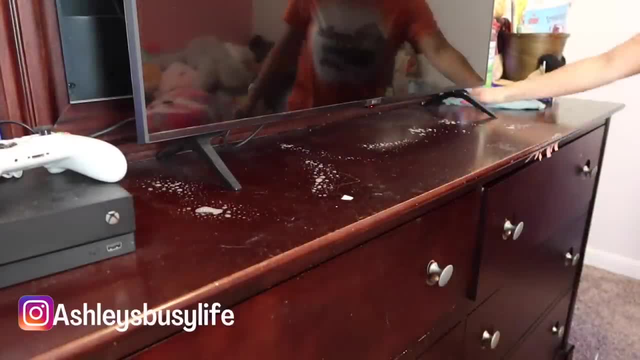 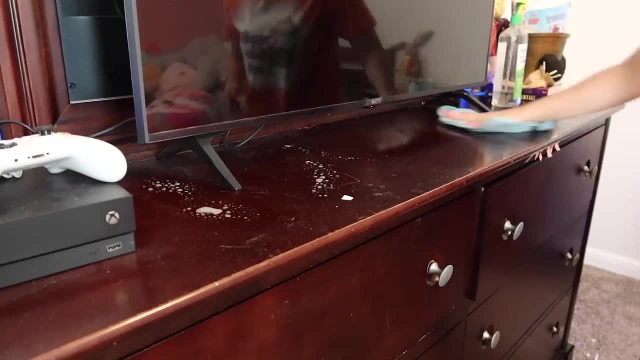 And that is just to kind of open up the drawer And then we can kind of open up the door. We also have this little drawer that is a little bit more of a work of art for us to kind of notice and sort of fill it out. 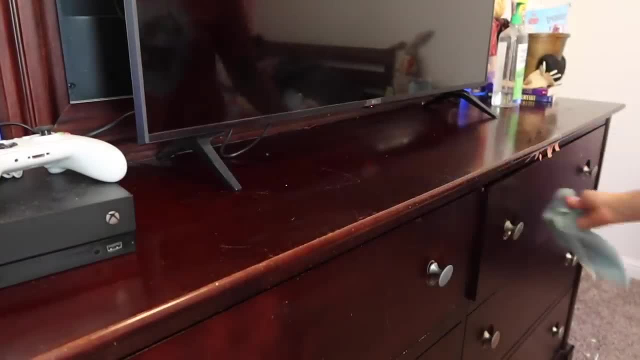 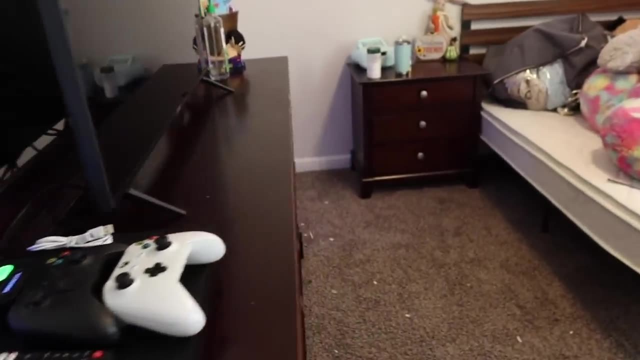 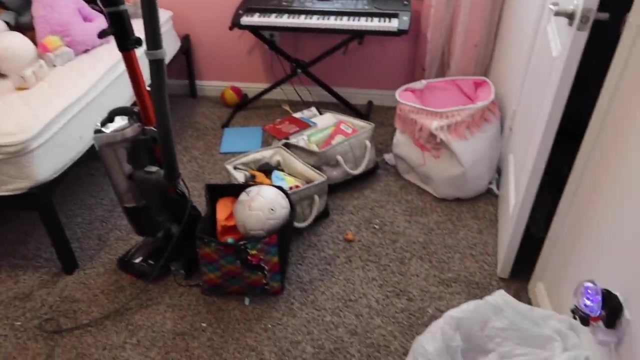 So this is a little shelf that we are like I'm going to be looking at. I'll see if we can find something we aren't looking at And then we can. you know, at so far The sheets are done being washed, but we're going to pick back up after I pick the kids. 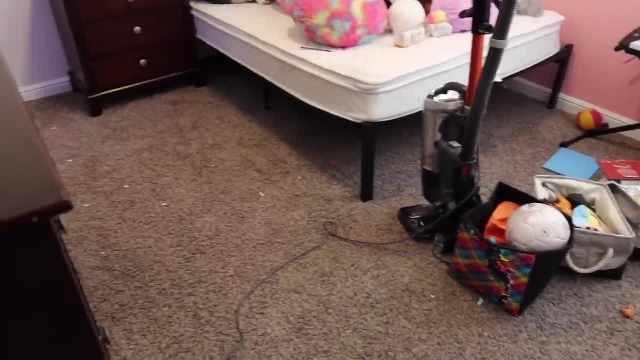 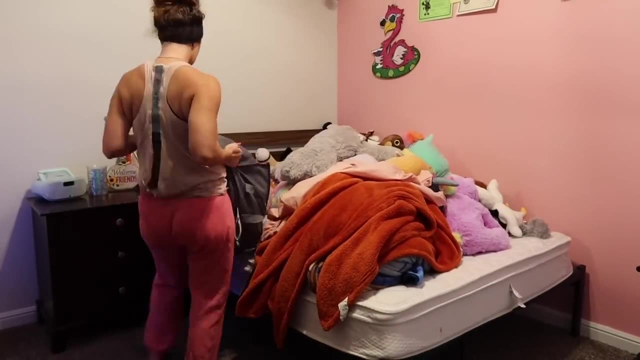 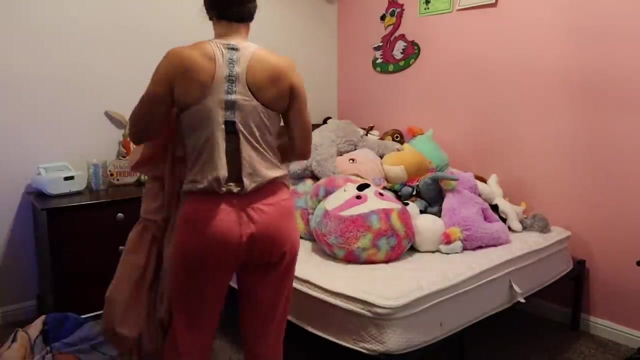 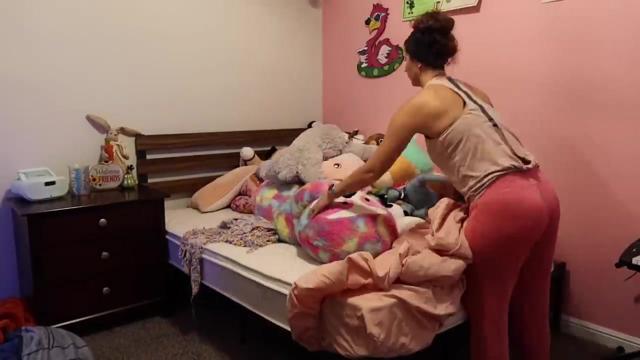 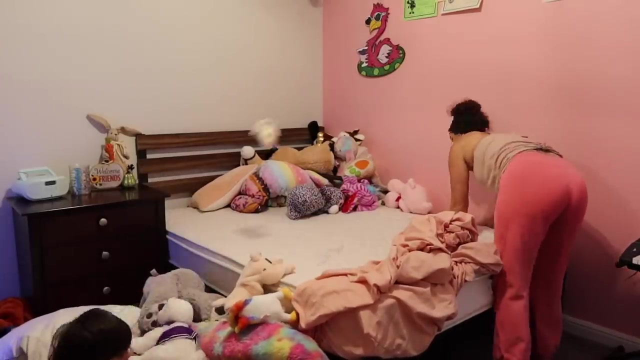 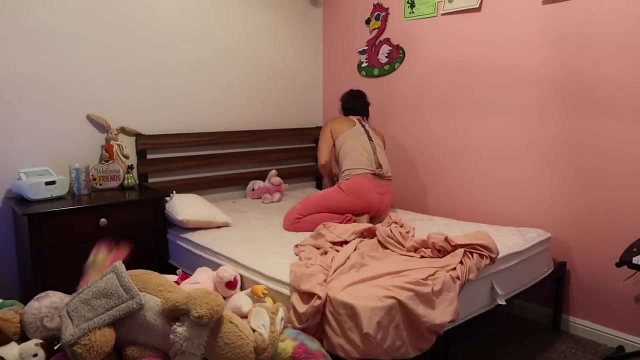 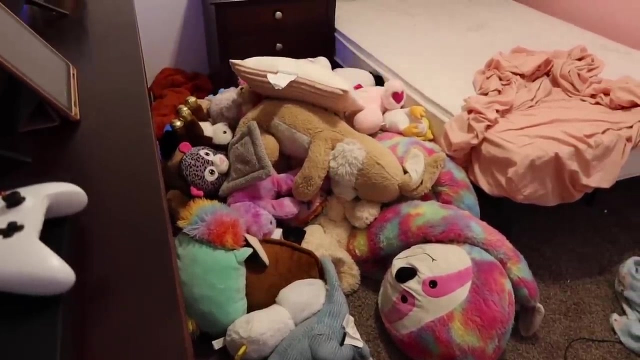 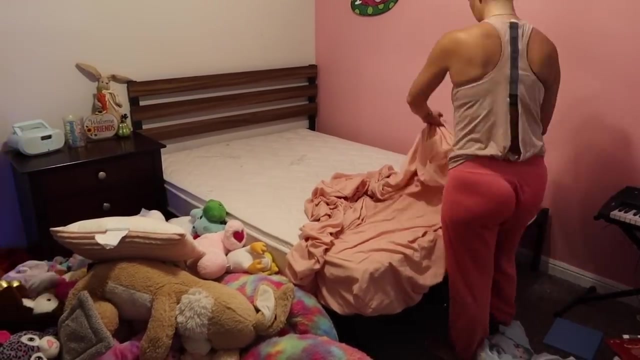 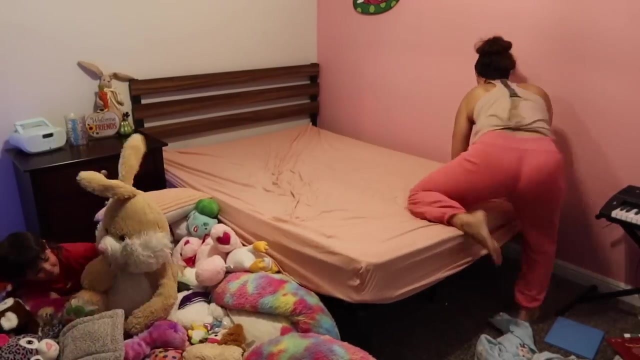 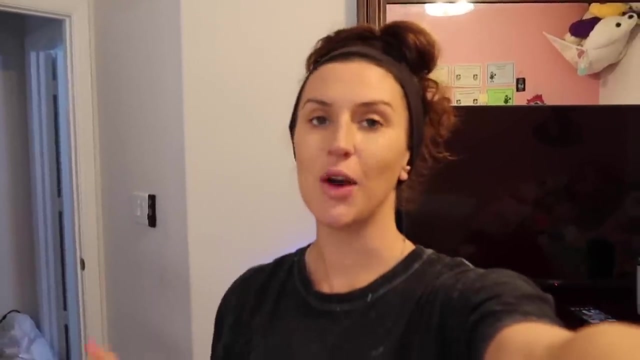 up from school because it is now time to go get them. This is a much bigger job than I thought it was going to be. There's all of Adrian's stuffed animals. That is insane. All right, you guys, it's now day two and I'm gonna try to tackle this. get it done. I'm actually. 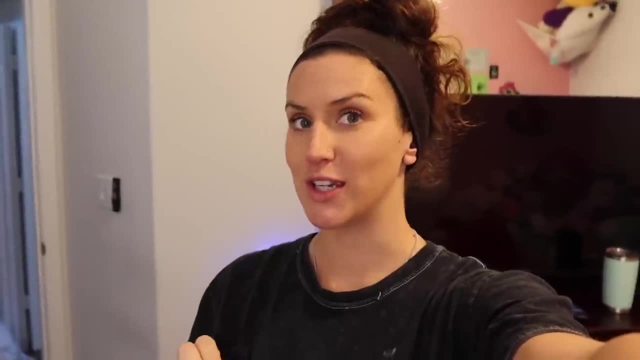 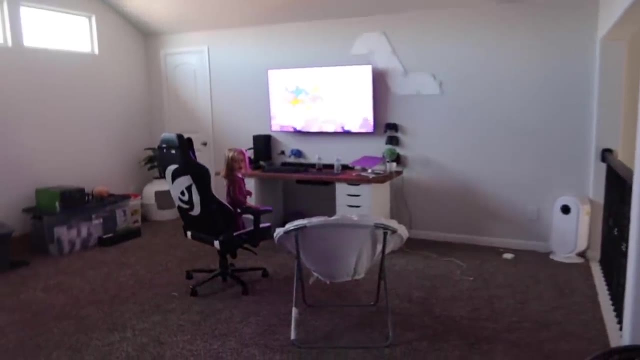 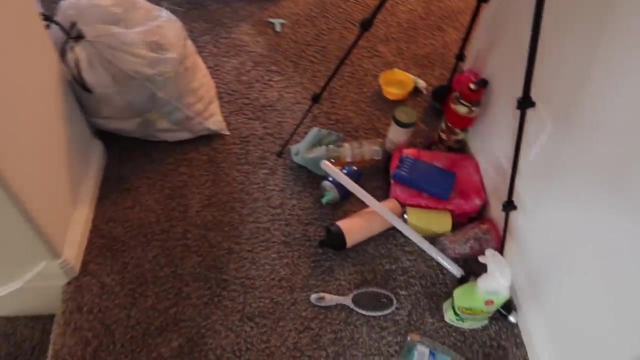 watching my friend's daughter again today. so I have two toddlers that I'm trying to distract while I accomplish this, So I have them set up in here Watching some baby shark. Ethan's in the chair, you can see his little feet, So let's get it done. I left everything yesterday, that way we could pick up exactly where we left. 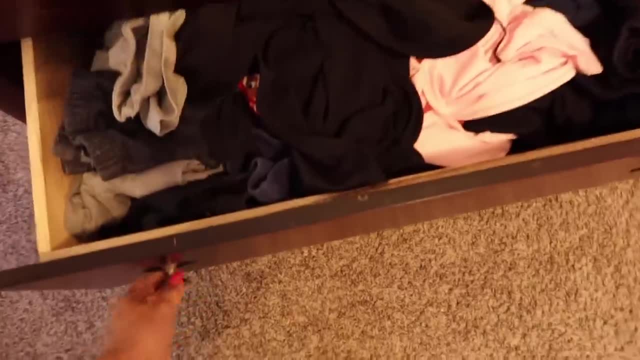 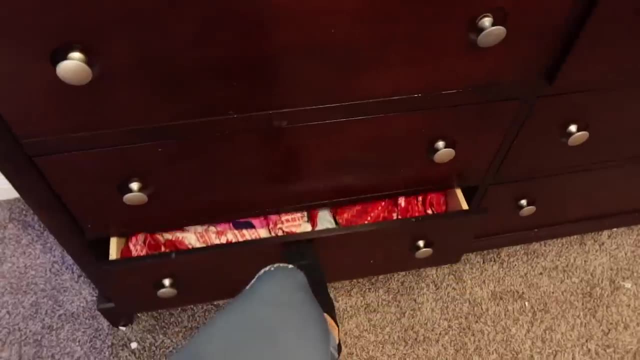 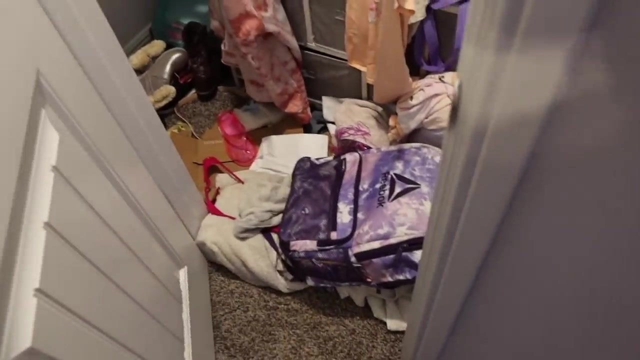 off. So what I want to tackle today is the drawers. As you can see, they're very unorganized, so I just want to organize her clothes for her, go through them, make sure there's, you know, no holey ones or anything like that, and then we're gonna get to. 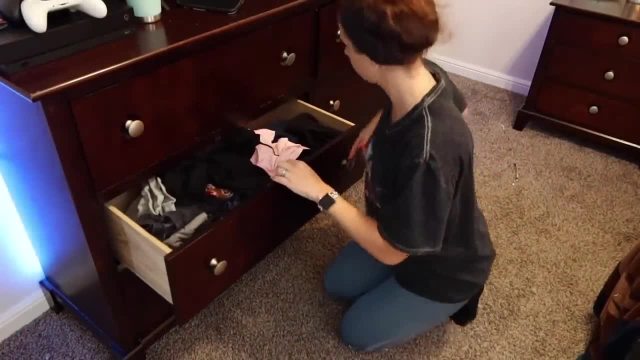 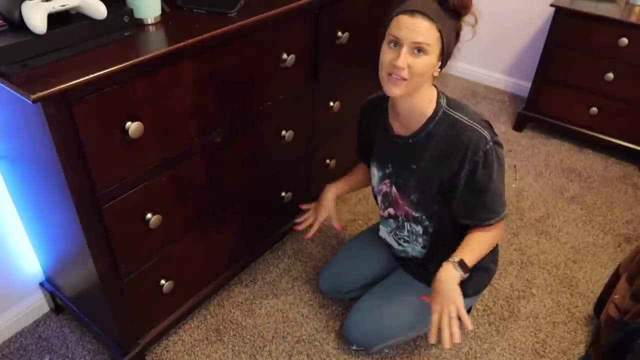 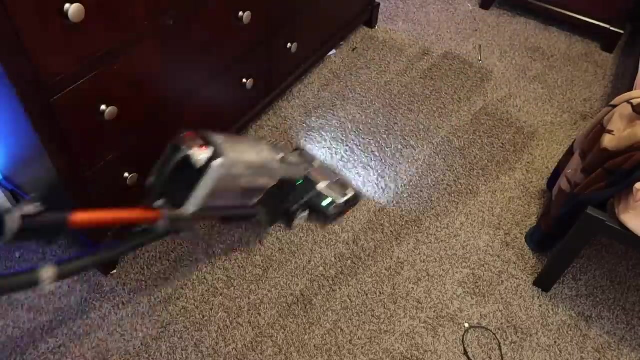 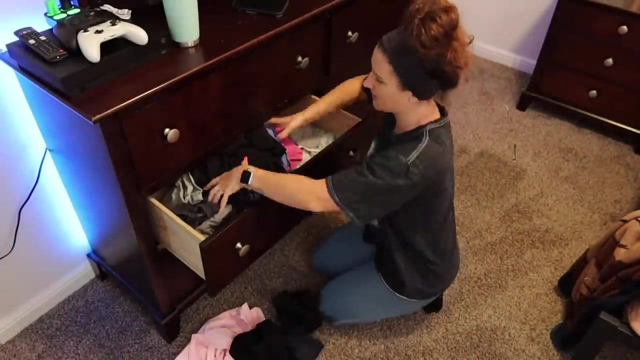 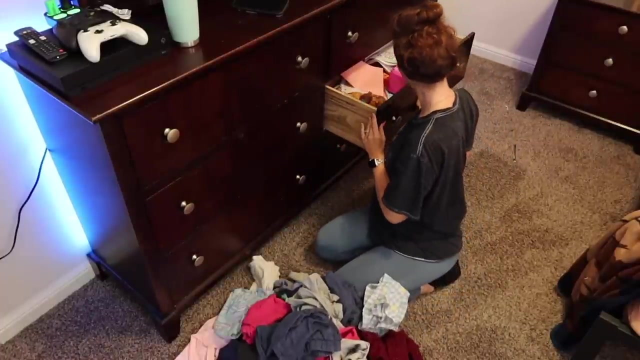 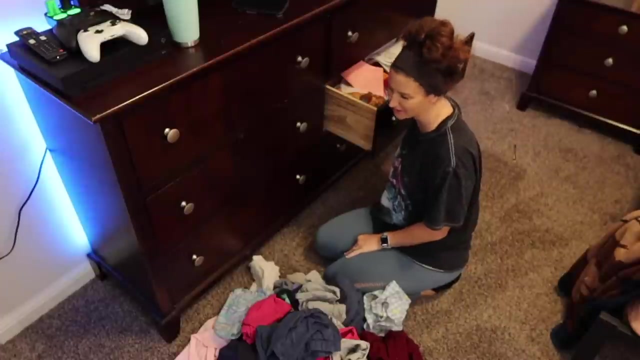 this closet. actually, before i pull all the clothes out, i'm gonna vacuum because her floor is gross. i can't believe. i live in your thoughts. i think about you all the time- morning, evening and midnight. such a wonderful delight y'all. she has another drawer of junk. i did not know that. we're gonna do her clothes first and 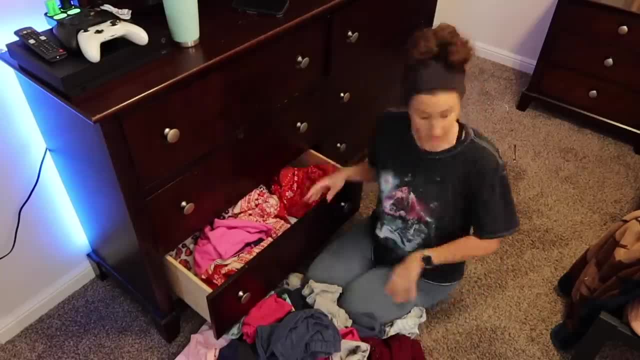 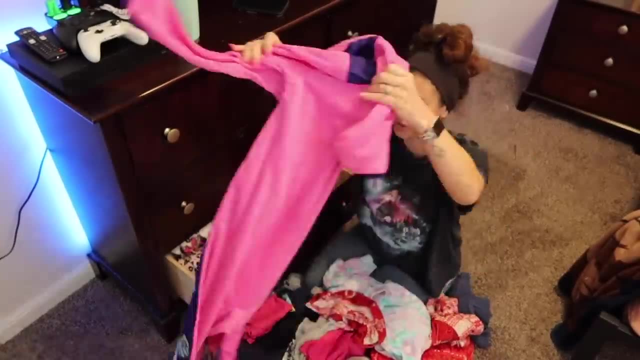 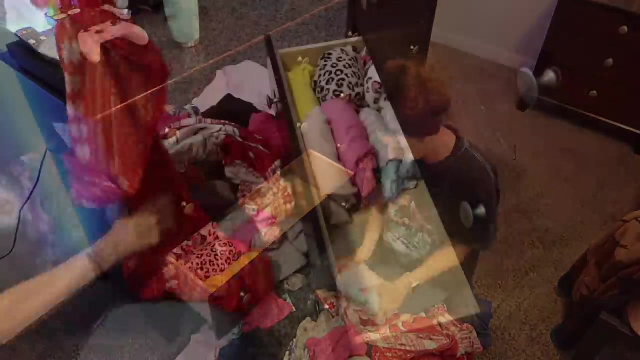 then we'll do that. i do try to do the konmari method for folding. i'm not the greatest at it, but i do try to do the konmari method for folding. i do try to do the konmari method for folding. i'm not the greatest at it, but 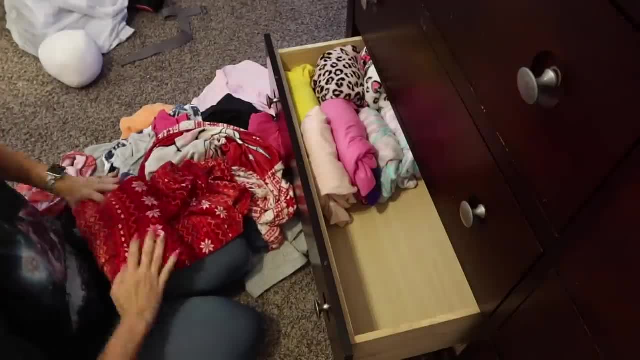 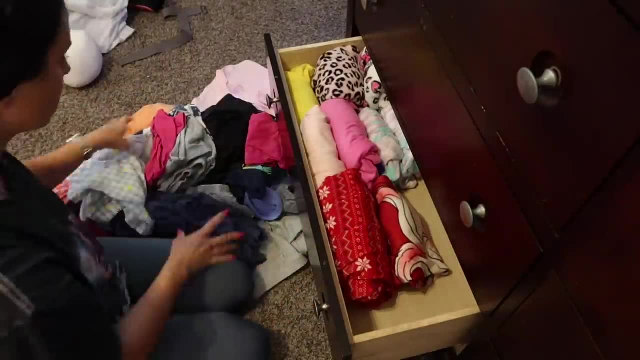 think it makes it so much easier for them to pull things out of their drawers. obviously it doesn't last that long, because adrian's the one that puts away her own clothes, and she'll start by trying to keep up and like, do the same type of folding, but eventually it becomes a mess, like it was when. 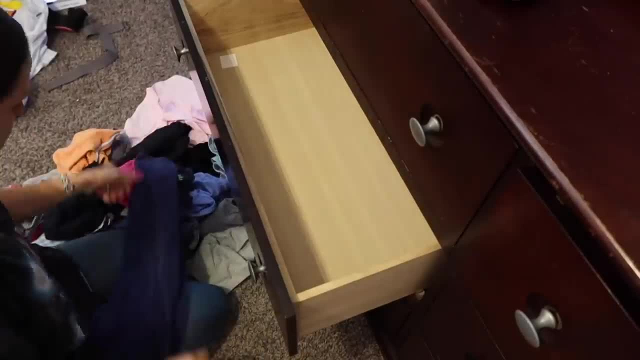 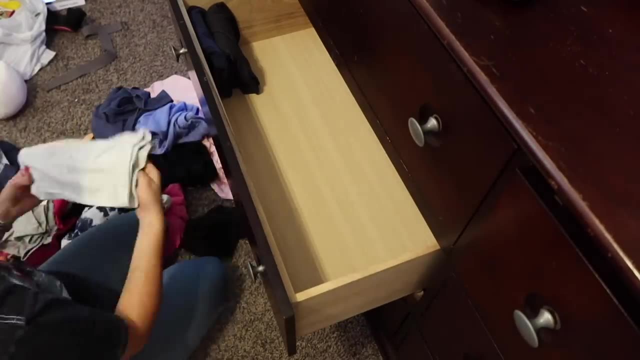 i got started, so at the end it does look really nice. i love the konmari method, especially for my clothes, um, and for little kids clothes, where when you're the one that's, you know putting the clothes in and taking the clothes out. it does make it so much more easier. i definitely recommend folding. 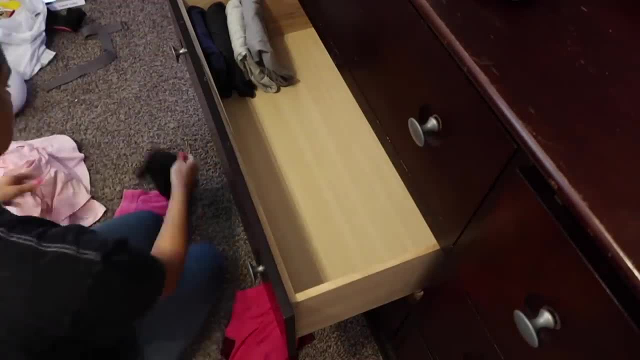 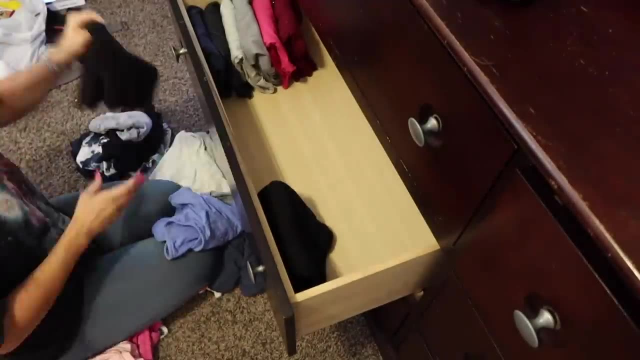 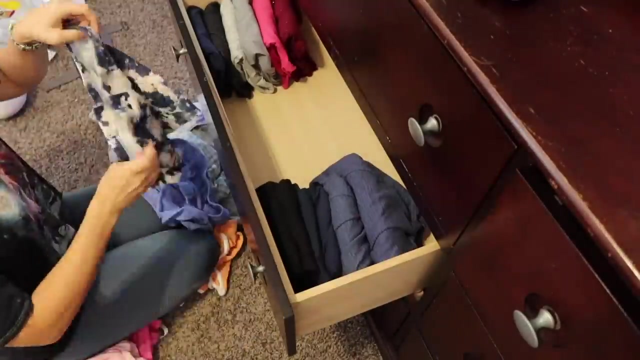 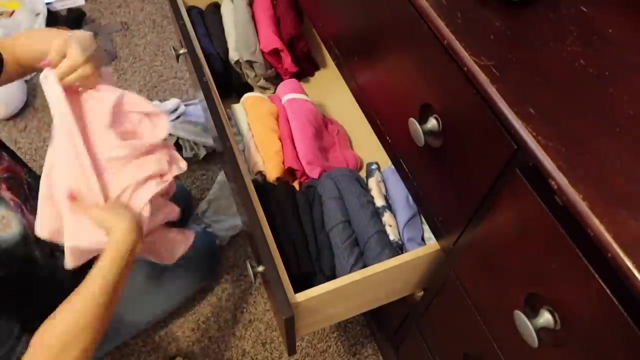 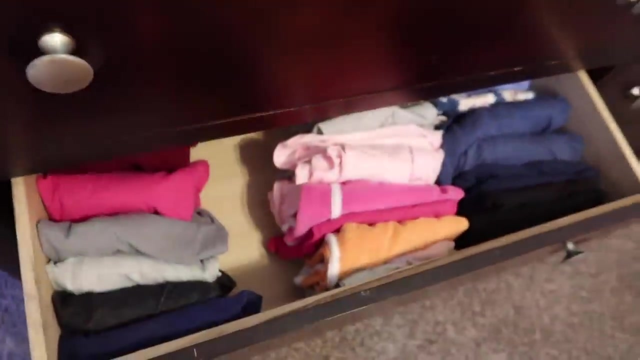 that way, especially when you have teeny, tiny kids with their little small clothes. as we hold each other tight, you're the rose in a garden and it shows, if i'm honest, you're the leaves. these drawers look so much better. i try to do the konmari method as best as i can, so these are her. 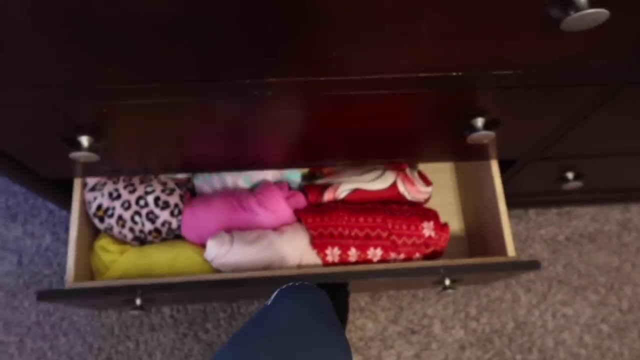 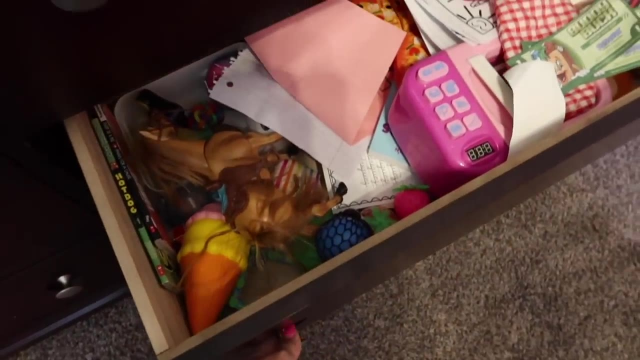 pajamas. these are her leggings and shorts. y'all know she lives in leggings, she does not wear jeans. and then her bottom drawer is her underwear and bathing suits. so we're not going to do that, but we are going to go through this drawer. i did not know she had another one of junk. 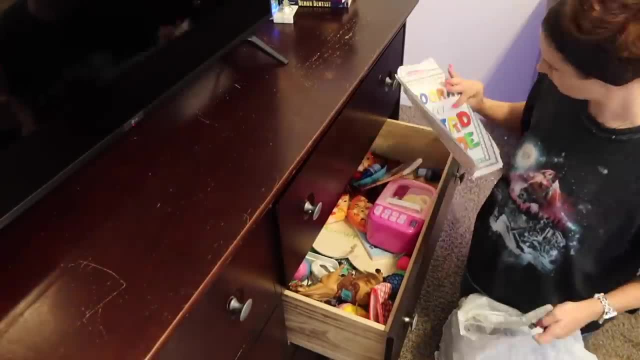 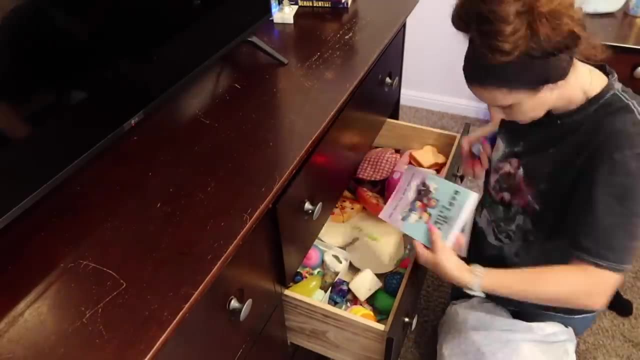 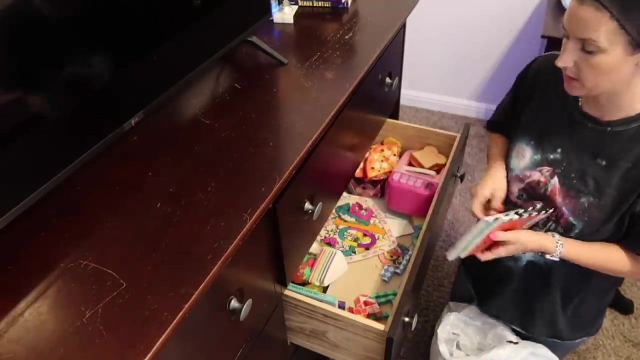 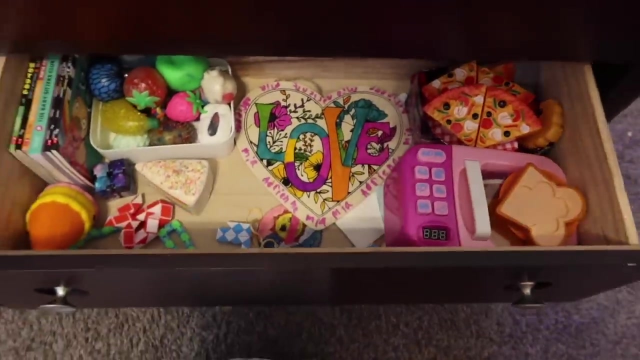 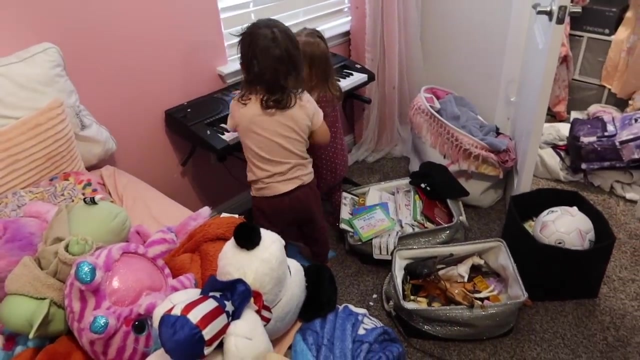 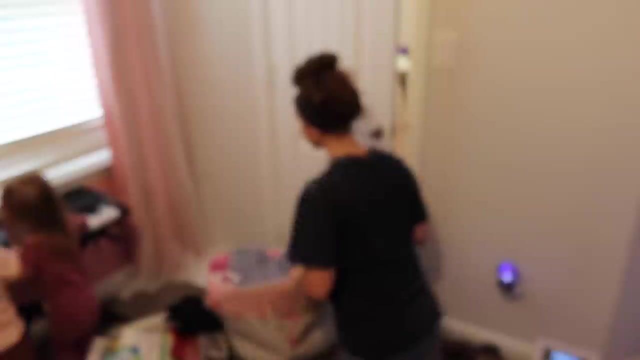 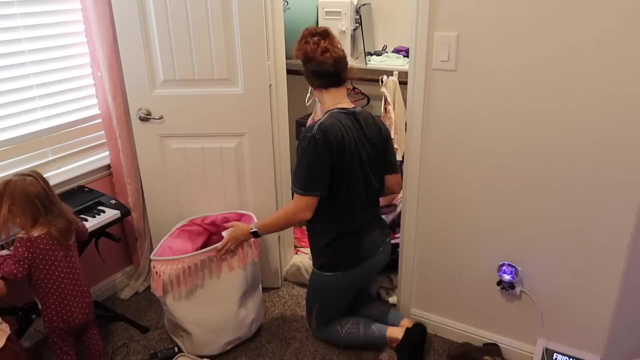 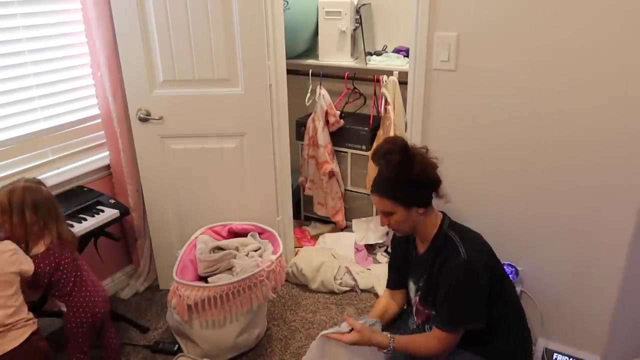 so she kinda had organization. so i just pulled out the trash, left it how it was, and we have some pianist over here playing me tunes while I clean. Just thought I'd leave a little clip in there for you guys so you can see what I. 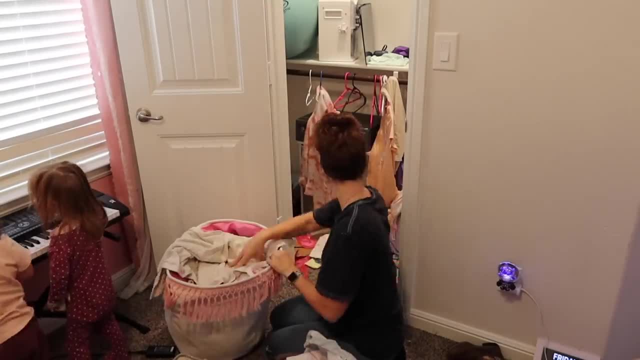 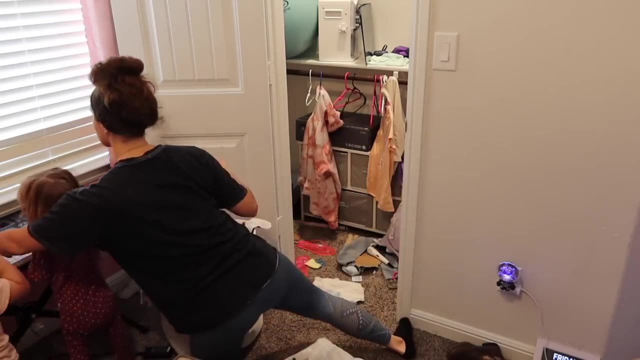 was listening to while I was cleaning. I was like, Oh my goodness, the piano. And then the kids whenever they turn it off and turn it back on. I don't know who designed this piano, awful idea. but whenever you turn it on, 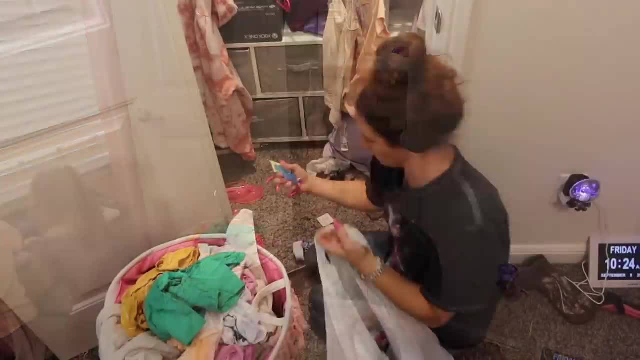 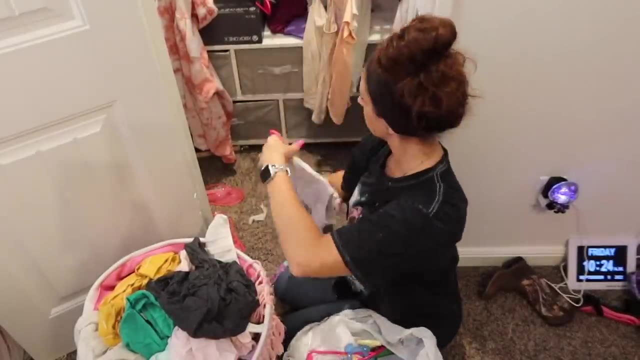 it starts off on the highest volume setting Like why? why would they create a toy where you turn it on and it's as loud as they could possibly go? So that's why I kept getting up, because I had to keep turning it down, because 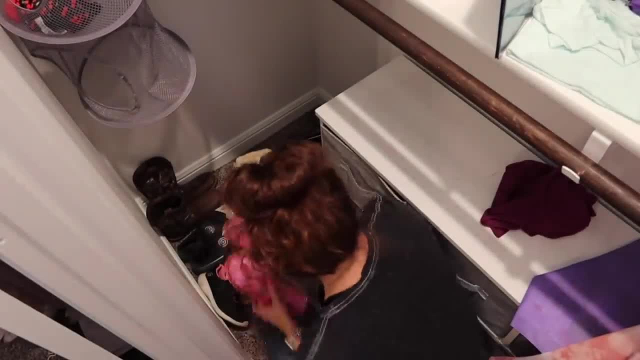 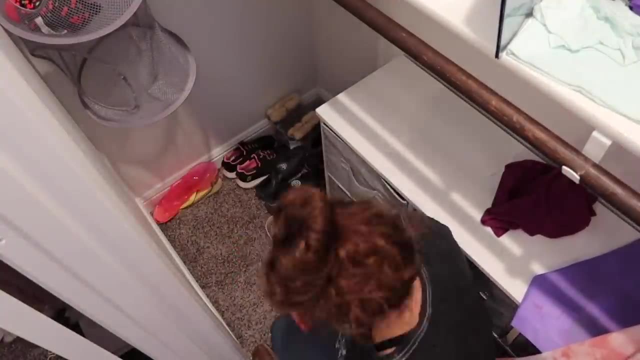 Ethan knows that if he turns it off and turns it back on it's going to be super loud again. So eventually I had to. I unplugged the piano because they kept turning it off and turning it back on And I was like, Oh my goodness, I can not. You're the only one who can get me so high. You are the only person in the world who can get me this high. So let's get into your car and go driving towards another town. Oh you know, I'm serious, I'm serious. 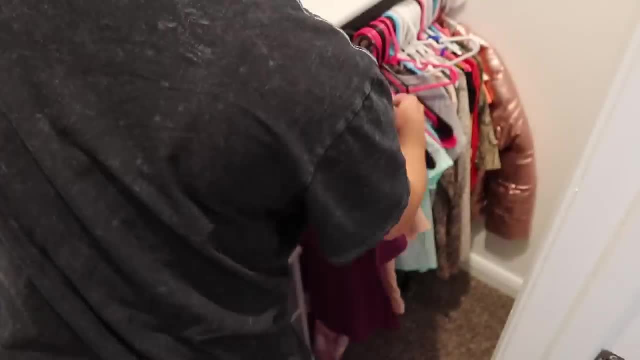 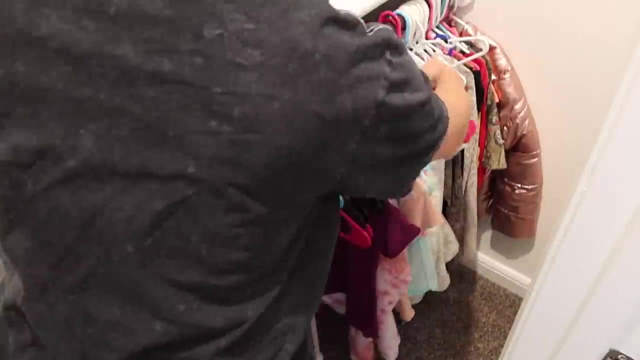 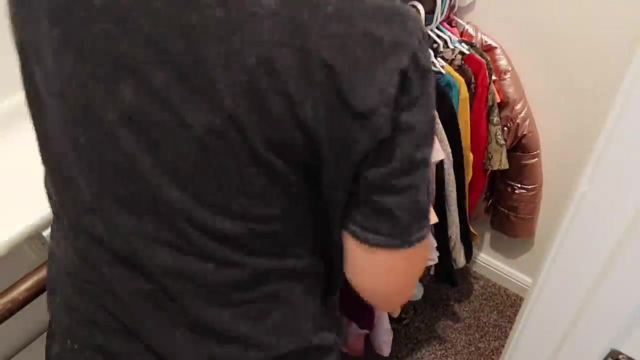 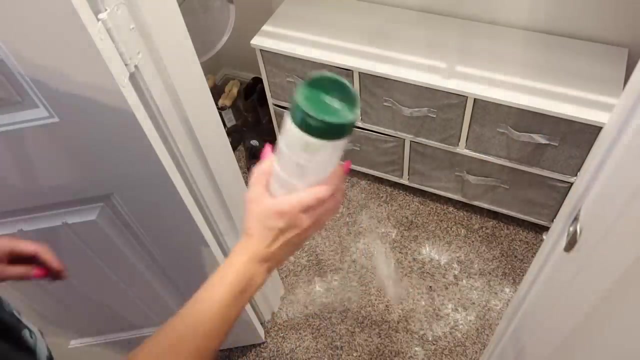 I will keep you all to myself. Oh, you're so mysterious, Mysterious, I can't keep my hands to myself. I'll walk across the room, Show you. ask if you want to be when the sun goes down, Cause you're the only one who can get me so high. 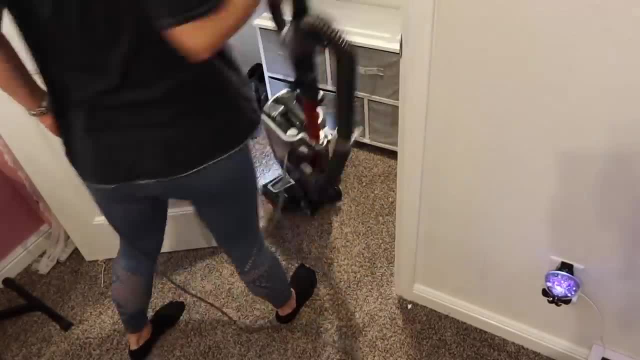 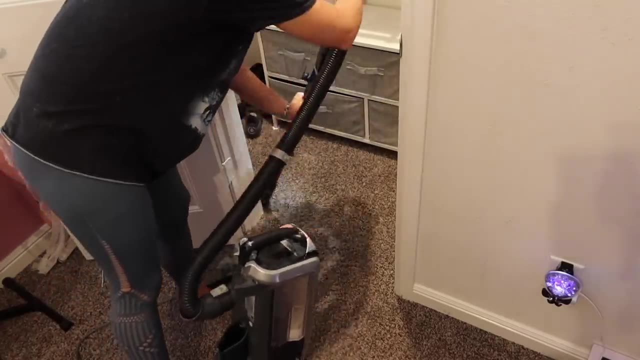 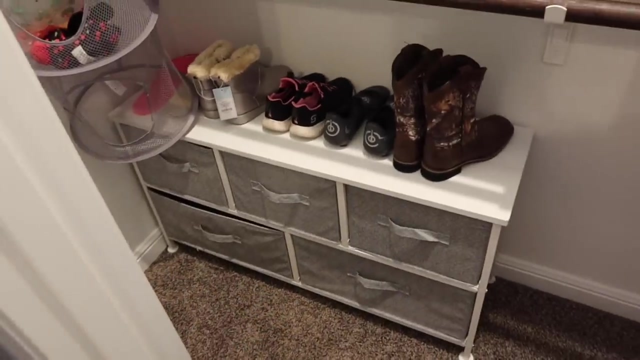 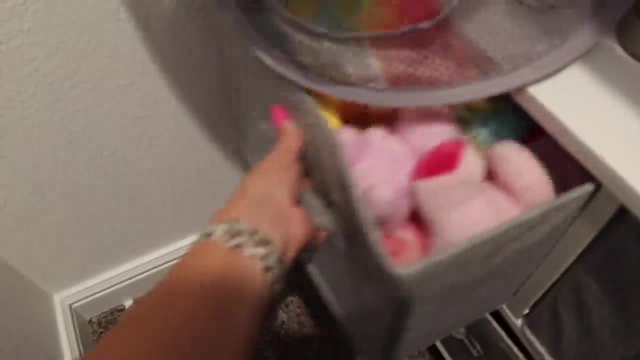 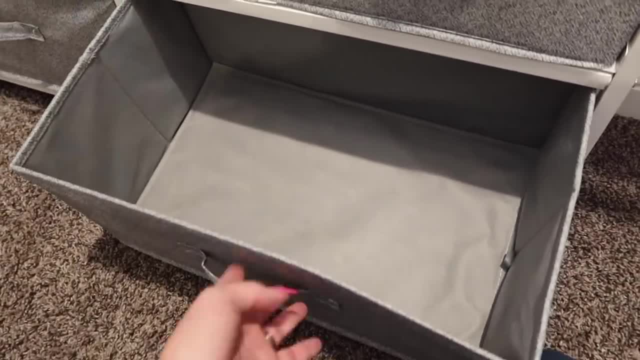 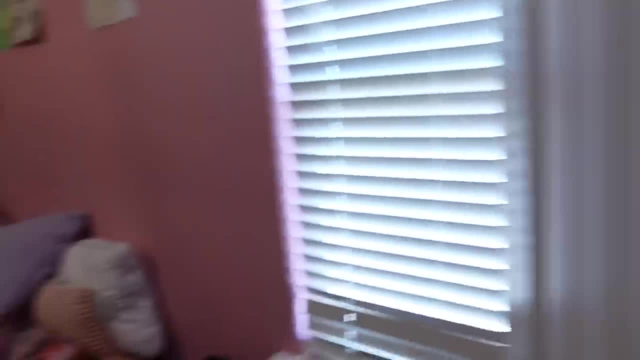 So she has this one free. I'm going to try to put some stuffed animals in here, and she has this little hanging thing, So I'm going to fill it up with some smaller stuffed animals, just to help get this bed a little less cluttered. 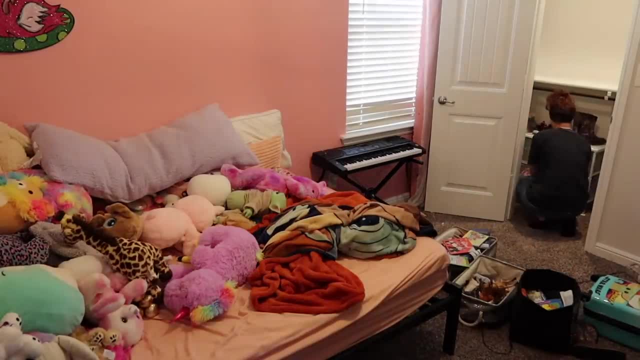 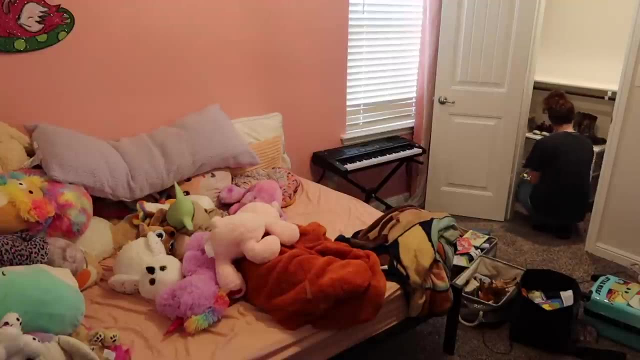 But I hope it's going to fit. I've got a scooter That's going to give you a little bit more space, So I'm going to put it in this little box and I'm going to hide it right here So you can put your toys in this little box. 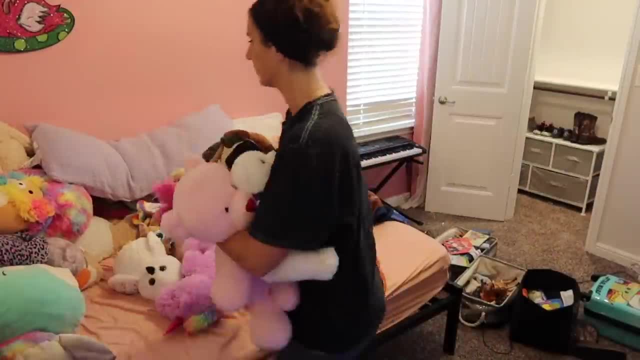 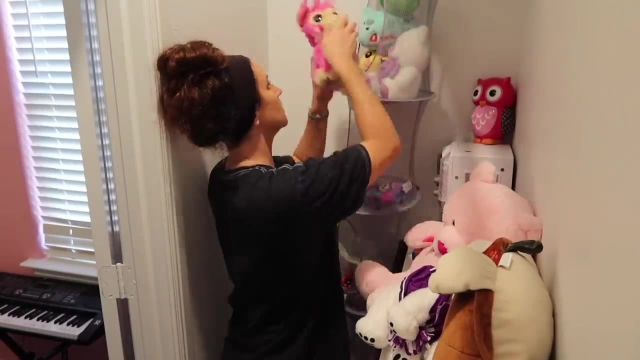 You can even put your dogs in there. You can put your cats in there. You can put your pets in there. I'm going to put my cats in here and make them sleep on my bed, So you can put your toys in there. 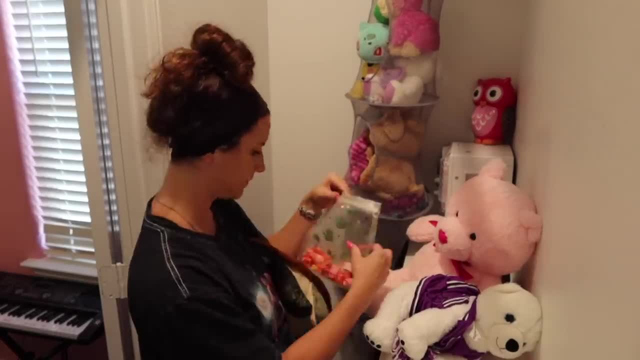 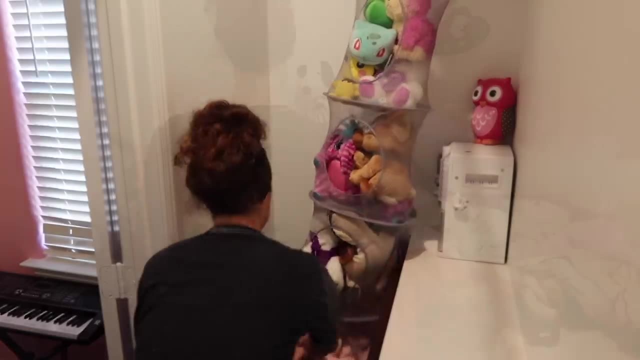 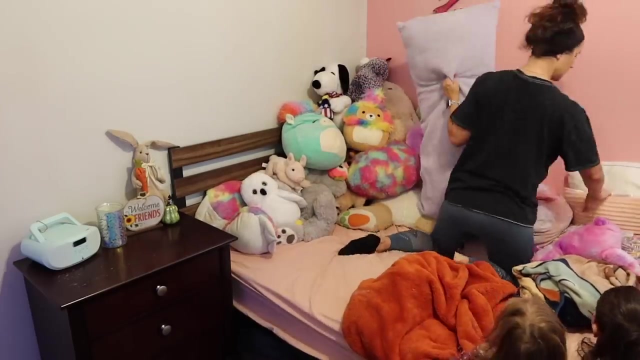 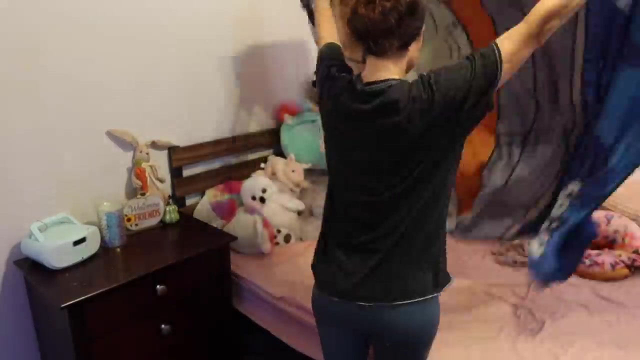 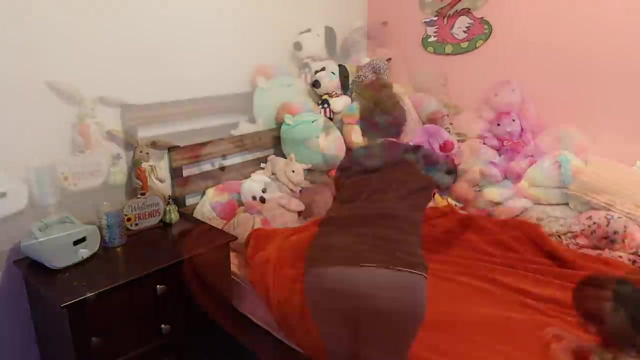 You can put your dogs in there. You can't have yourself stuck here. This is about as good as it should be, As good as her bed is going to get. It's still a lot of stuffed animals, but better than what it was.